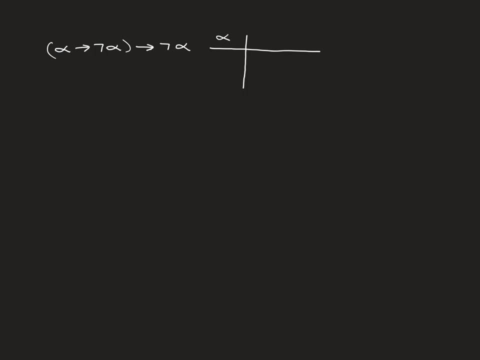 If it weren't a tautology, you know, if it weren't the case that, for whatever true or false values, whether alpha is true or false, this is going to come out as true. If it weren't that case, then we would need to know more about what alpha consisted of. 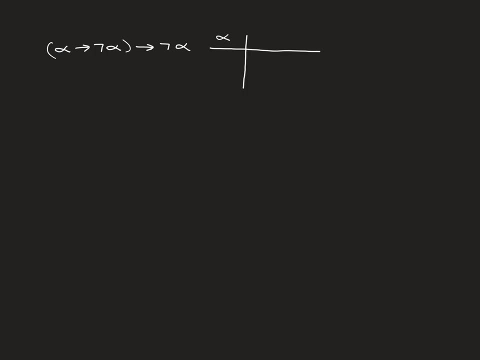 Because, for example, if alpha was a tautology itself- ie no matter what combination of true and false you ascribe to the propositional variables that make it up, it's always going to come out true- then it wouldn't matter that this statement- if alpha was false, comes out as false. 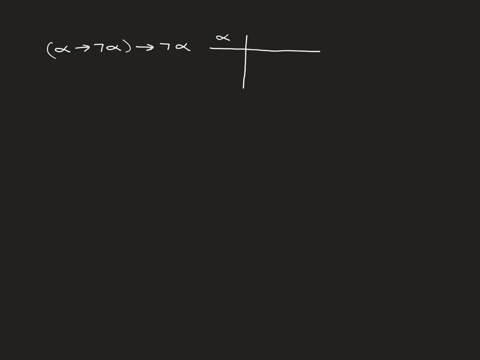 because alpha is never going to come out as false. So we'd only have to look at the true case And then if the true case came out as true, then it would overall be a tautology. But in this case it's going to come out true for both values of alpha. 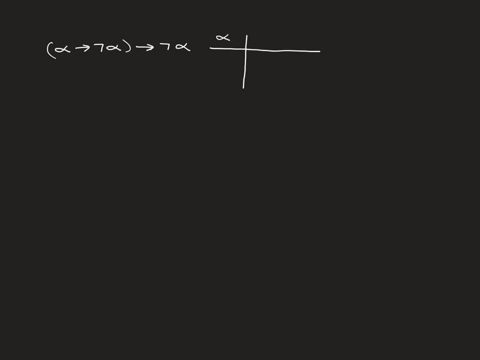 So we don't need to worry about what alpha is It's made up of to establish whether this thing is a tautology or not. So for the two different values of alpha, then true or false, not alpha. we can then write nice and easily. 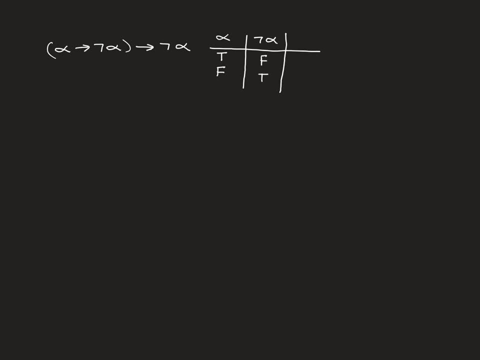 So for alpha being true, not alpha would be false. For alpha being false, not alpha would be true. And then we can think about: alpha implies not alpha. What's the value of that going to be? So when alpha is true, not alpha is false? 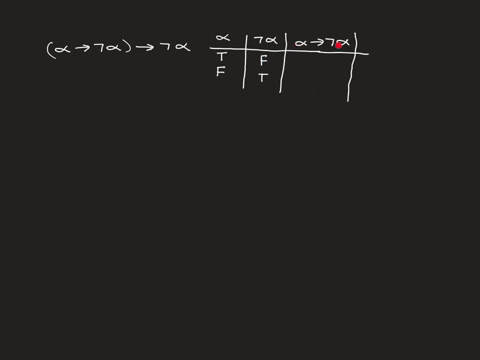 So the implication is then wrong, because it's not true to say that when this one's true, this one is true, So it's false in that situation. But for the second one, remember: expulso quodlibet from false follows anything. 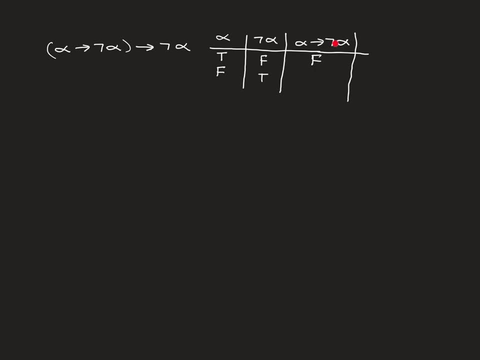 So because alpha is false, it's fine that this one is true. It is a true implication in that case, because this implication says: if this one is true, this one is true Because this one was false, it It has nothing to say about it, so it's vacuously true in that case. 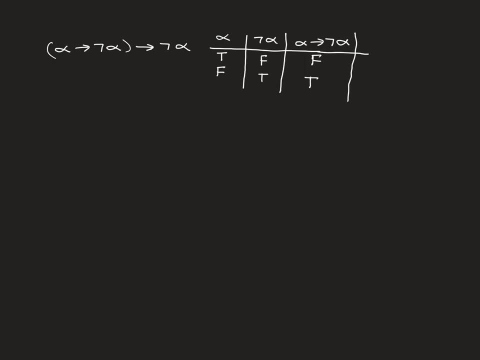 That's something that you have to get used to when you first see logic. But the more you see of it, you realise that it's the best way to define implication, the way implication works. And then let's go further. So alpha implies not, alpha implies not alpha. then 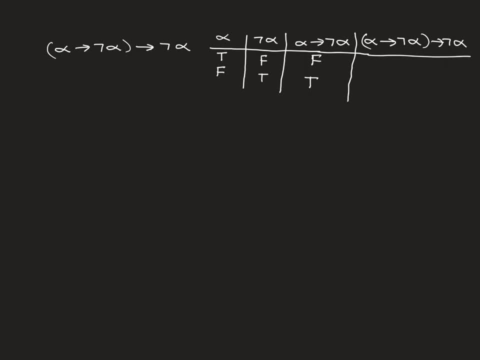 So the whole thing- and we're hoping this is going to come out as a tautology- So in this line then: so this one is false, so we've got false here. So then we don't need to even go any further, because the moment you have false in the antecedent of an implication, 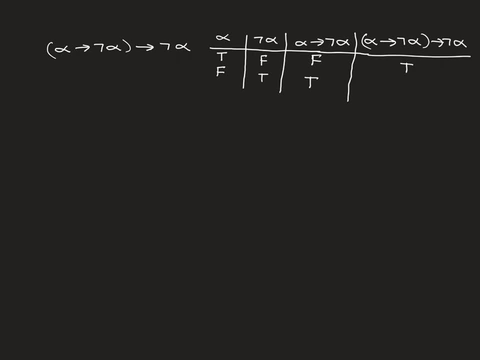 we know that that's going to come out as true, So the implication is true in that case. Here it's true. but then this one also is true, So we've got true implies, true, so it is also true in that case. 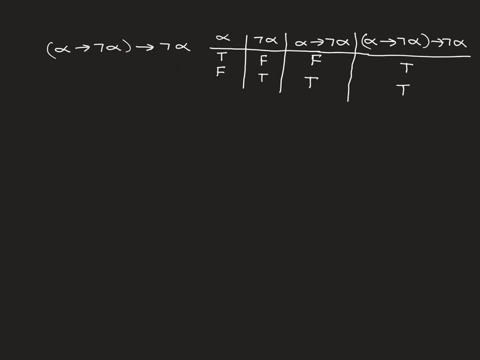 So we've therefore shown with this truth table that this formula here is a tautology- Excellent. So we now want to do A four more Hilbert-style proof. So for this, I should probably concretely tell you what the structure I'm working in is going to be. 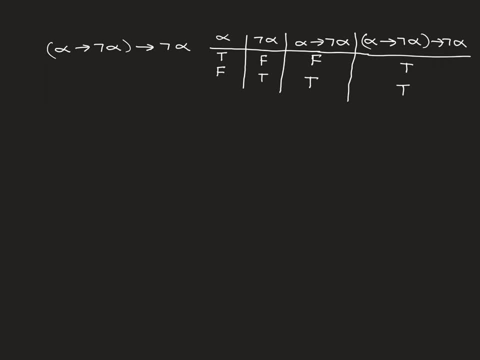 So we're working in propositional logic, zero-order logic, and we have a bunch of propositional variables. potentially, We don't need to know how many propositional variables. We then are going to only have two logical connectives. So I'm going to get rid of and or 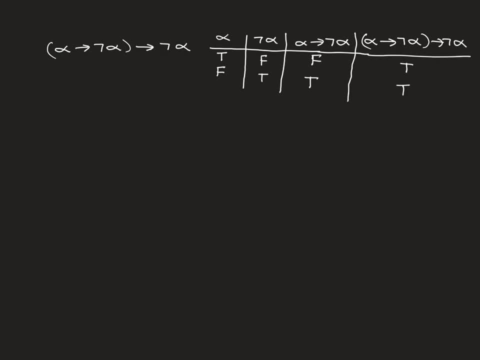 We don't need them and I'm certainly not going to have biconditional implication. The only symbols I'm going to have are not and implication. So my set of all formulas is going to be everything that is generated from the propositional variables, with these two logical connectives. 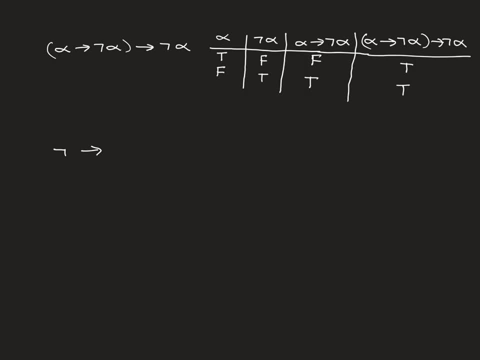 Then, now that I've got that, I need to tell you what my proof system is going to be. So we're going to have a Hilbert proof system, And there are multiple different Hilbert proof systems. The thing that they all have in common is that they have bigger reliance on logical axioms. 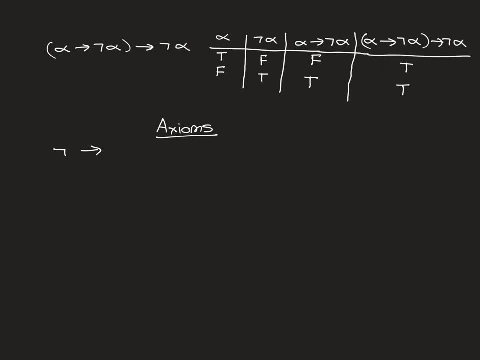 and then they usually in zero-order logic. in propositional logic they usually only have one rule of inference, And that's in contrast to different types of proof system where they have much more rules of inference. So in Hilbert-style proof systems in propositional logic you usually only have modus ponens. 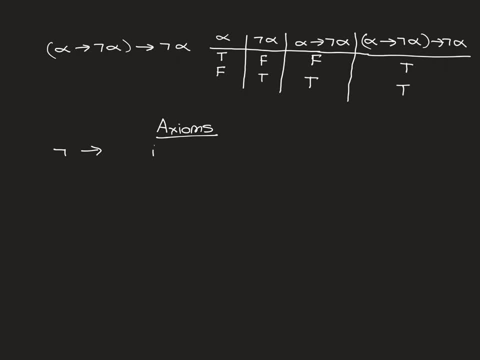 And a bunch of logical axioms. So I'm going to give you three logical axioms. They are quite standard, but especially the first two. Pretty much most Hilbert systems that you see defined in different textbooks always have the first two in common. 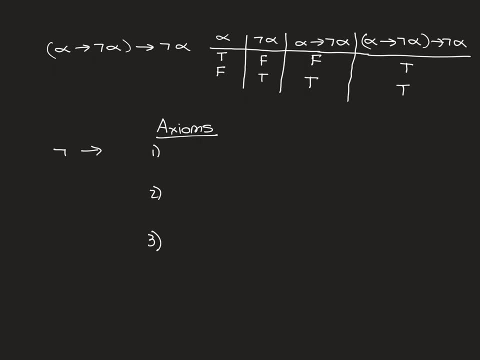 The third one is the one that can change, and sometimes they get rid of it altogether and just have the first two. But I'm going to define the third one in a certain way, and it's quite a common way that you'll see it defined. 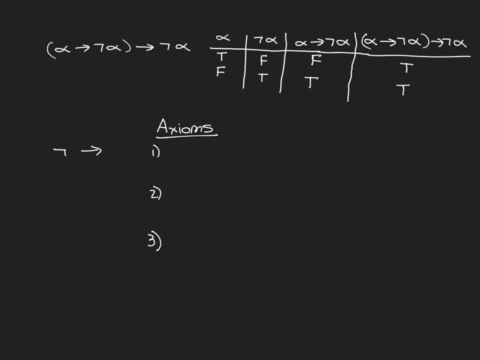 So the axioms, really The axiom schemes they are. they define a bunch of formulas that we're allowed to use and take as axioms in our proof, And it's all formulas that fall into the form that is specified in these free axiom schemes. 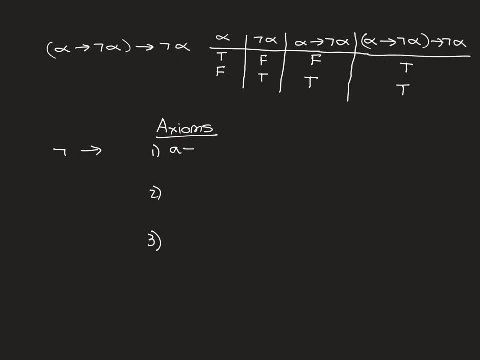 So the first one is anything of the form a where a isn't necessarily a propositional variable. it could be a propositional formula. So a implies, b implies. Oh, and just a few warnings about the way this video is going to work. 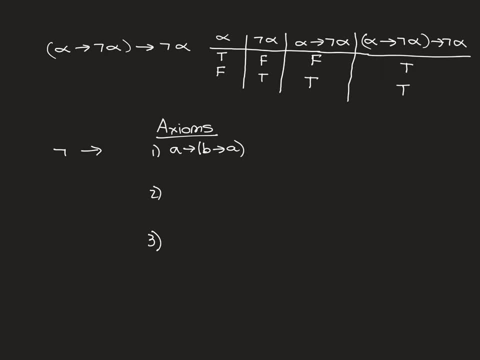 So, firstly, this formal proof that I'm going to give of this formula is going to be quite long. It's the proof that I came up with for this formula. I thought about it for a very long time and I came up with this from looking at other things on the internet to get inspiration. 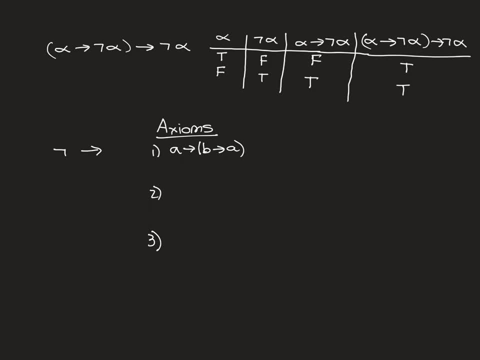 But that comes with a warning, which is that it's long and it might not be the most efficient way to do it, And if it's not, if there is some really simple way to do this, I do apologise. The second warning is that this isn't going to necessarily be a polished performance, so at some places I might go wrong and have to correct myself. 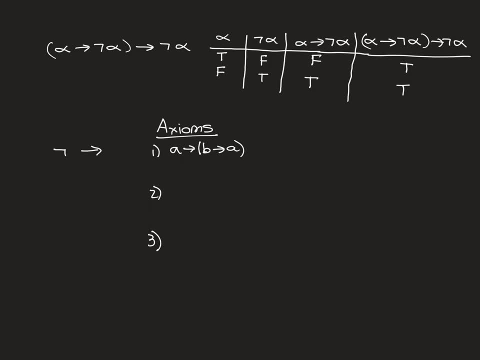 If the video is uploaded, don't worry, I do eventually get to the right answer. I wouldn't have uploaded it if eventually, I end up with the wrong answer. So I will get to the right answer, but I might have to pause and think if I'm going down the wrong track- and I can see that I'm going down the wrong track. 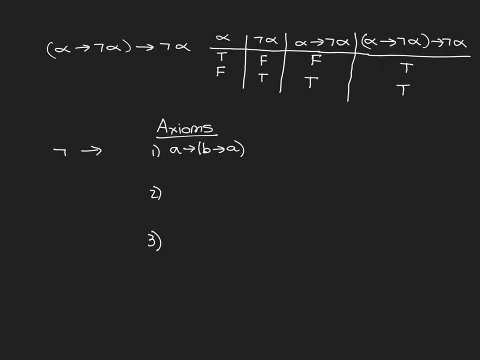 Um, and The other warning was that I'm going to be a bit lax with my brackets. So you know, strictly speaking up here, we should have had an extra bracket there And strictly speaking here we should have an extra bracket. 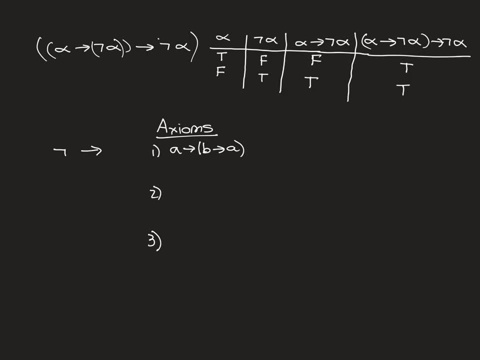 Oh, in fact there should be even more brackets. We should have brackets around the knots here. I'm not going to do that. I'm going to put in enough brackets that the meaning is clear. So I'm going to put brackets where it's really, really important for meaning. 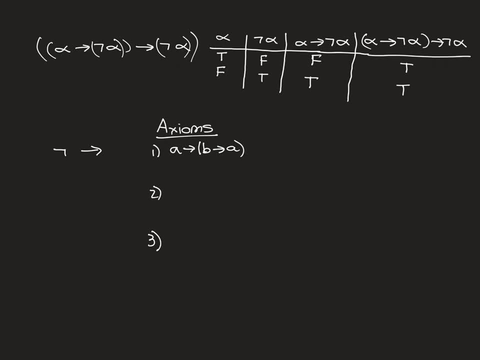 I'm going to drop brackets where there should be some formally, but it doesn't really need them. It's still got a clear meaning. It's still got a clear meaning without them. So I'll be a bit lax with brackets. So I'm being a bit lax with brackets here. 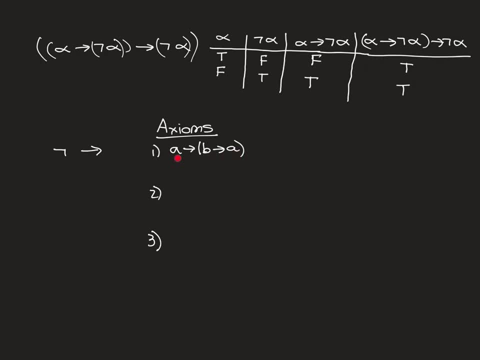 So anything of this form, A implies B implies A. that is axiom one or the first axiom scheme in our Hilbert proof system. And again, A and B are not propositional variables, They are formulas. So for example, I could take this whole formula and stick it in there as A. 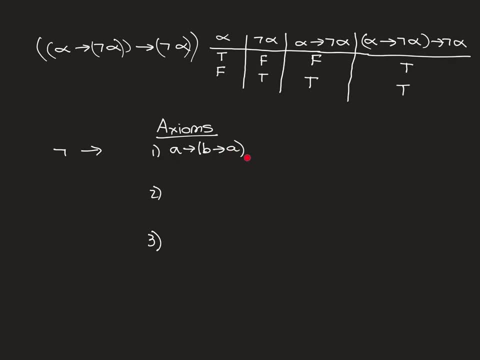 As long as I put the same formula here as here, that falls into the set of things from my things, from my well-formed formula set that we're going to have as our axioms in our Hilbert proof system. And, as I say, this first axiom scheme, well, firstly, it covers a lot of different things. 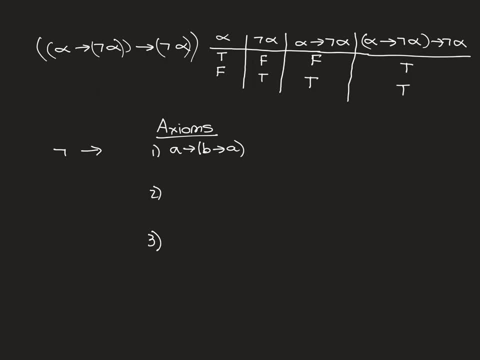 You know there's going to be a whole bunch of things that are now axiomatic formulas, But it's also very standard in Hilbert systems. I think you'll pretty much always see it in any Hilbert system- that first one. 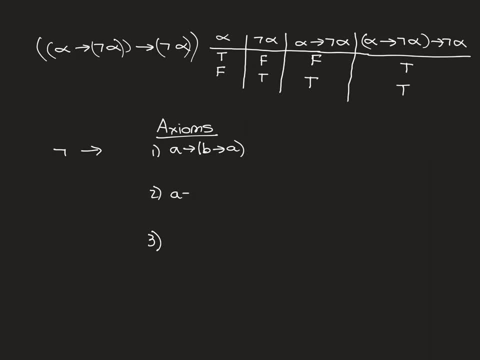 And the second one's also quite standard. So it has A implies B, B implies C this time, And we do need another set of brackets: Implies A implies B, implies A implies C, And another set of brackets there probably to make it absolutely clear. 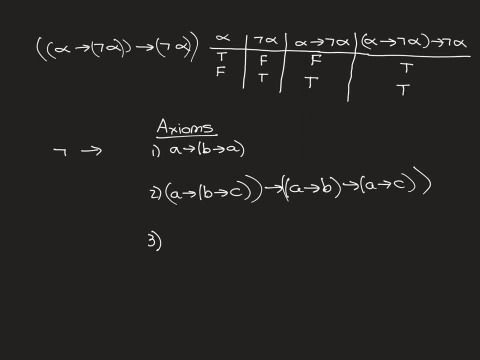 So this says that if it's true that A implies that B implies C, then it is true that if A implies B, it is true that A implies C. So again, A, B and C are not necessarily propositional variables. 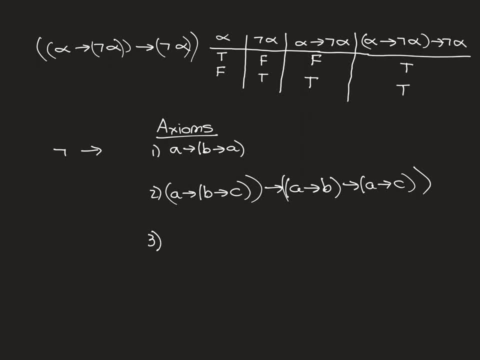 They might be propositional formulas. As long as you have the same one here as here and here and the same one here as here and the same one here as here, then you can have any propositional formula you like. So anything of that structure is now in our set of axioms as well. 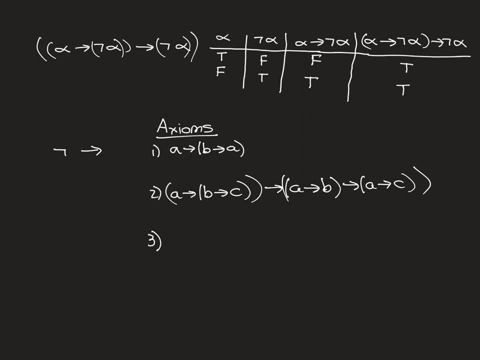 So that's a whole bunch of propositional formulas. Indeed, an infinite bunch of propositional formulas is captured by each of these axiom schemes. And then finally, axiom 3, which, as I say, in different textbooks you'll see it done differently, slightly differently. 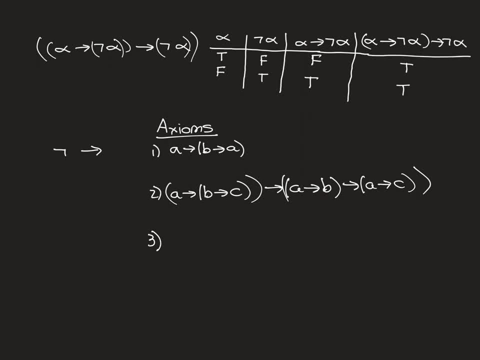 They're often equivalent, might be different. You know, some of these Hilbert systems may well actually end up having slightly different properties. where they change this axiom, Other ones, where they change it slightly, it might end up being equivalent. But this is the one I like. 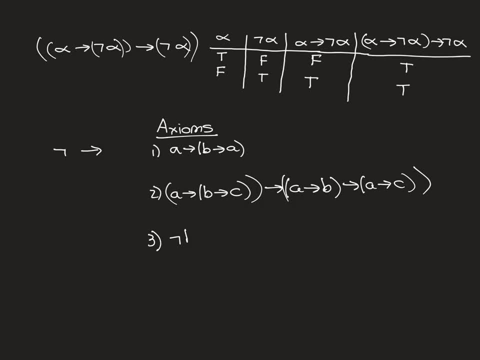 I think it's one of the most commonly used ones. So it is that if not B implies not A, then this implies that A implies B. So it's kind of modus tollens or contraposition backwards. So it says that if not B implies not A is true. 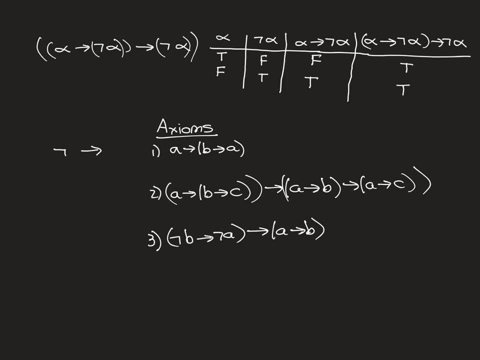 then A implies B is true. So again, A and B can be any propositional formulas you like. Any formula that's overall of this form is now an axiom and falls into our set of axioms. So those are the things that you can do. 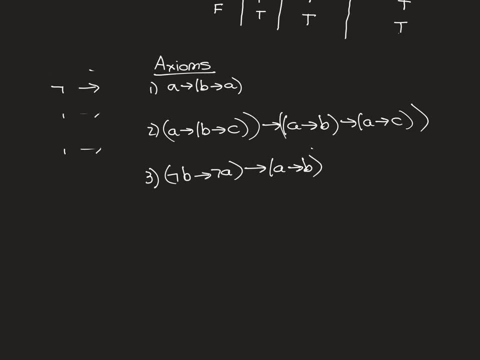 So those are the logical axioms in our Hilbert system. We've then got our one rule of inference, which is going to be modus ponens. So one of the most famous laws of logic, one of the most famous rules of inference. 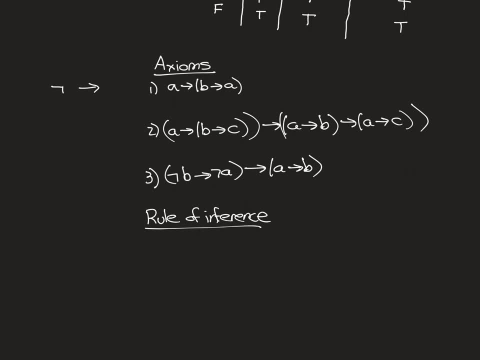 probably the most famous rule of inference, made famous, of course, by Socrates. You know, all men are mortal. I am a man, therefore I am mortal. That's modus ponens. So modus ponens is an operation, really. 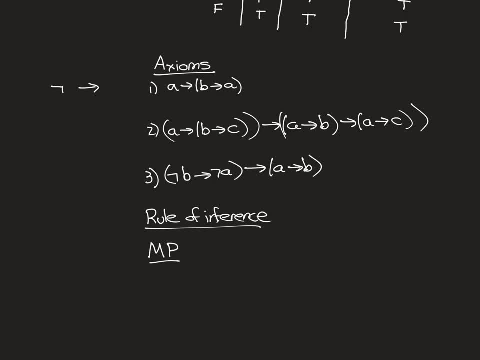 on the set of propositional formulas, except that you can't just combine any two elements together. For loads of combinations of two elements it's not going to be defined what modus ponens gives you. It gives you doesn't work. But for some specially chosen two elements 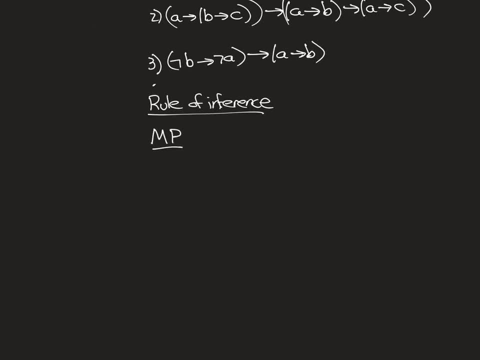 it will give an output. So it says that if you have a propositional formula alpha- let's say I'll go back to Greek- and you have a propositional formula of the form alpha implies and that should stick to Greek beta. 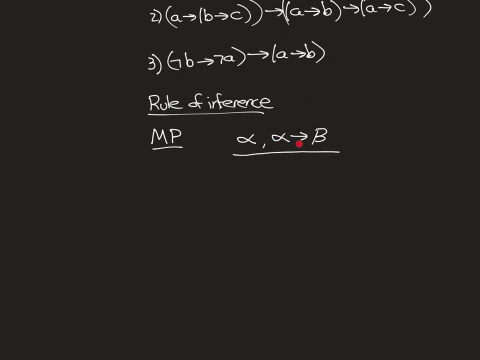 So that's, you know, one of the things that you are inputting, one of the arguments to your operation has to have the first argument in the antecedent position of an arrow, logical connected. So its form, its out of most form. 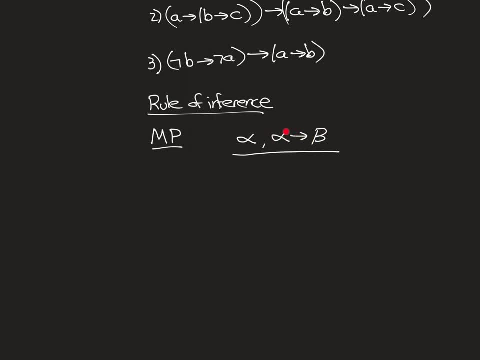 has to be that it's an arrow structure and the antecedent has to be your alpha, and only then will it actually spit out an output. So if you have alpha, and you have alpha implies beta, you can get beta from that. 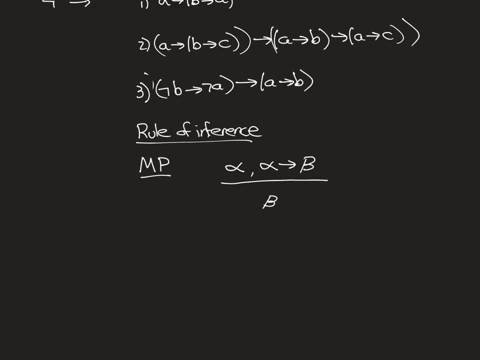 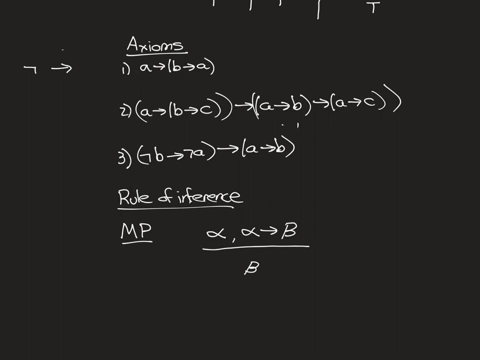 And things that are going to be allowed then in our formal proof are going to be in our sequence. that makes up the proof. we're going to be allowed statements that are axioms and then we're going to allow things that are obtained from previous things in the sequence. 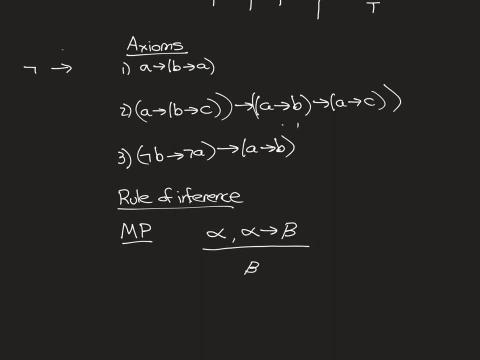 by applying modus ponens. So you'll have two things in your sequence previously, where one of them is the alpha and one of them is the alpha implies beta, and then you'll be able to add beta as the next element in your proof sequence. 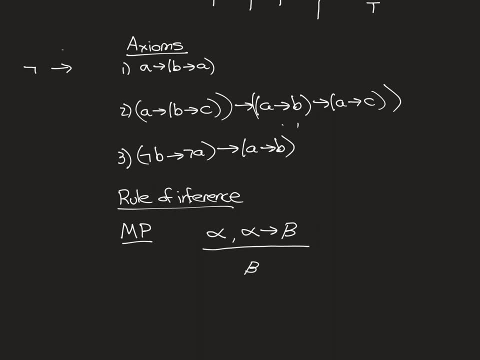 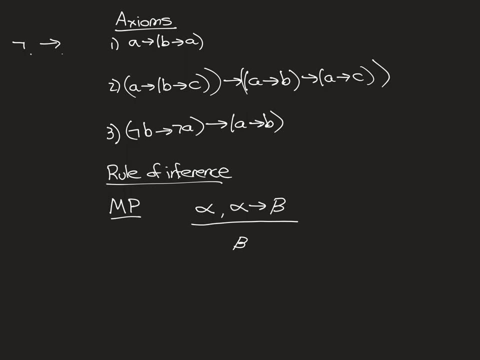 by applying your rule of inference, which is modus ponens, And that's how we're going to formally prove things in our system, With the axioms and with this one rule of inference, and we're going to have to create a formal proof sequence. 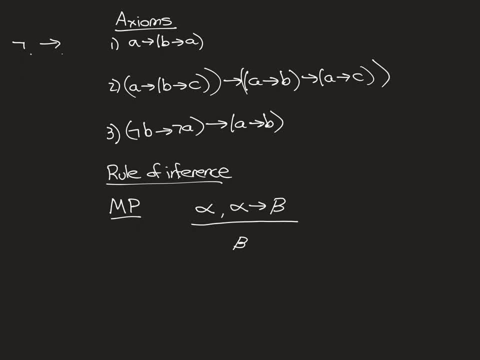 And we're going to try and do that, for alpha implies not, alpha implies not alpha. The one other thing that we're going to do is kind of a cheat, but it's a wonderful cheat And we're going to accept that. we know the proof of the deduction theorem. 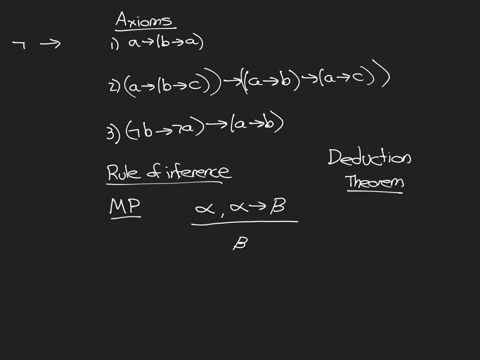 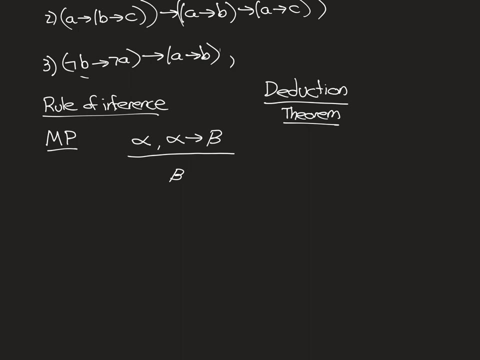 for this Hilbert system. So this Hilbert system does obey the deduction theorem and the deduction theorem is highly, highly useful. Apologies, It's getting late. So what does the deduction theorem say? So it says that. Oh, one thing that I haven't mentioned. 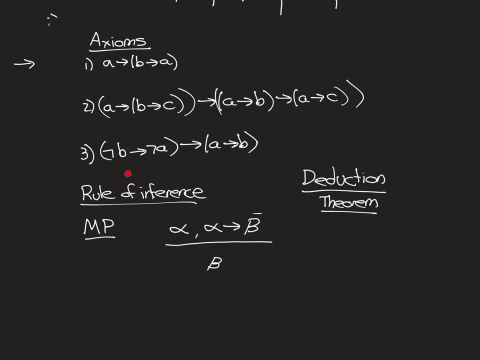 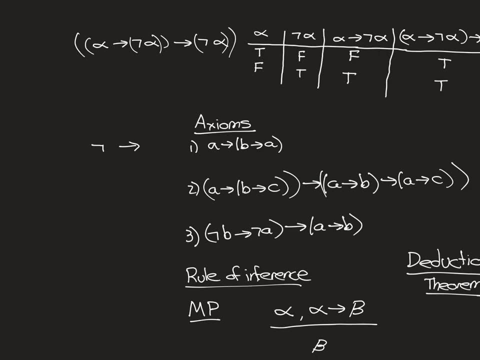 So this is proof from just axioms alone, And in this case this is a tautology and we can prove it from just axioms alone. But more generally, of course, when we're proving things, we might have assumptions as well. 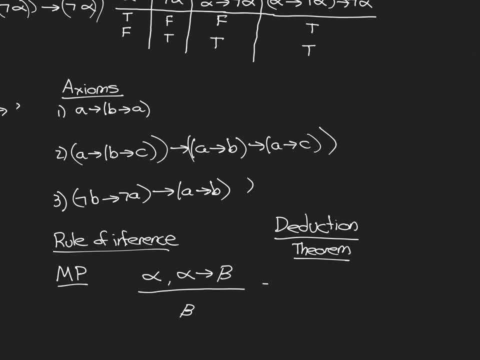 So we might have a set of assumptions, And when I'm stating the deduction theorem, I should include include the possibility that you have a set of assumptions. So if you have a set of assumptions, all that is is a set of propositional formulas. 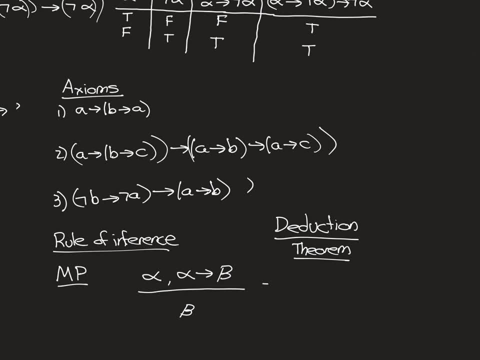 that you're also going to allow to be used in your proof sequence. So they don't need to be axioms and they don't need to be obtained from modus pollens, from previous things. You can just use them in your proof sequence. 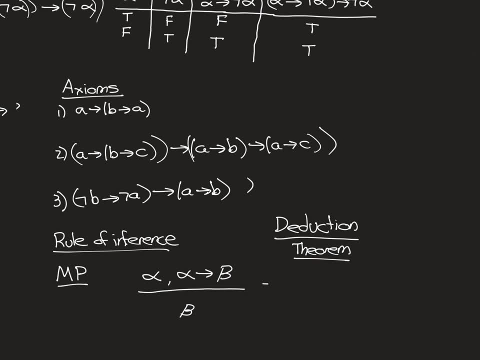 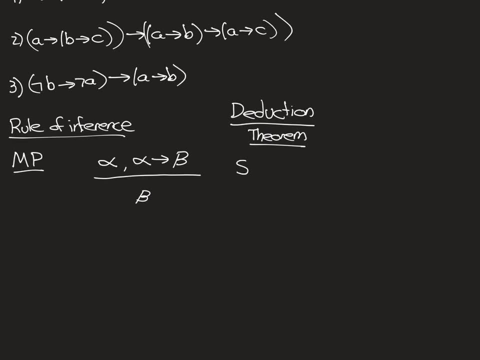 They're your premises in your proof, the things that you accept that are true but which aren't quite axioms. So the deduction theorem says: if a set of premises S with a further premise that I'll just call- and I'm overusing- alpha- 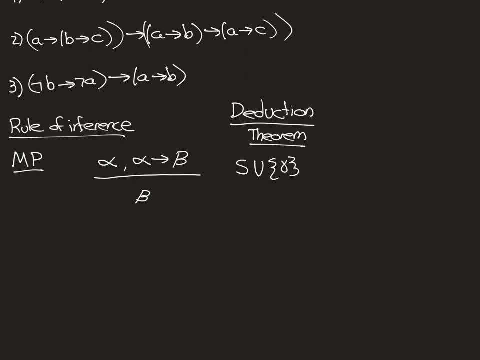 so we'll use gamma now, So S union gamma. So we put in this other premise gamma If that is able to prove. so this is the symbol for: is able to prove with our Hilbert-style proof If it's able to prove delta. 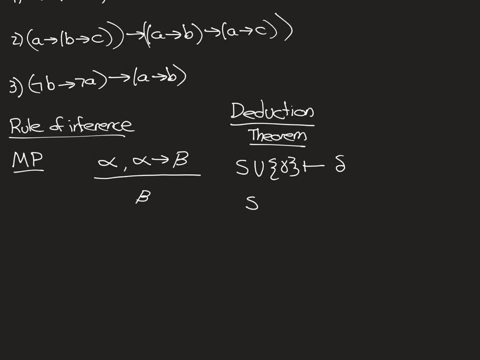 then if you just have S alone, S is able to prove gamma implies delta. So this is the deduction theorem stated. If it's the case that this is true, then this is true, And this is often really really helpful in doing these formal proofs. 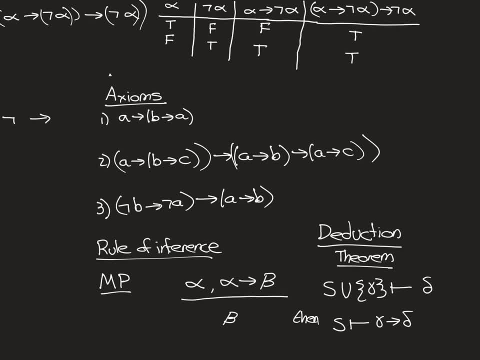 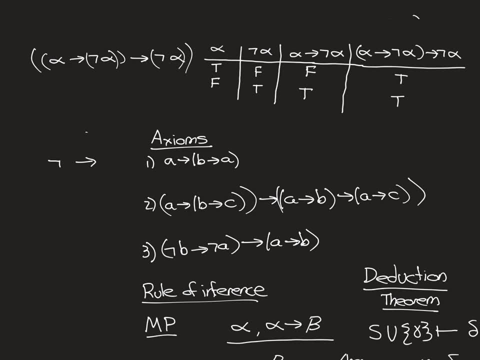 It's a cheat. basically Doing a lot of them without the deduction theorem is really difficult, And we're going to use the deduction theorem here because we've got an arrow statement here. So the way we're going to use it is we're going to say: 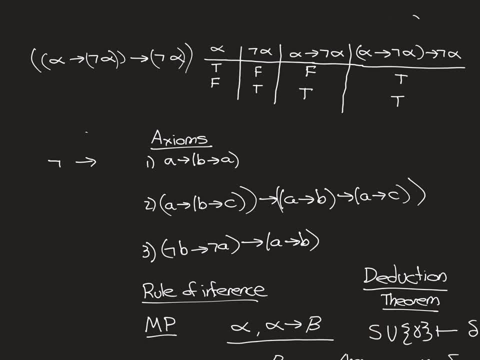 our set of premises is going to be the empty set. We're not going to have any, But then our gamma here is going to be this thing We're going to assume. alpha implies, not alpha as a premise, our one and only premise. 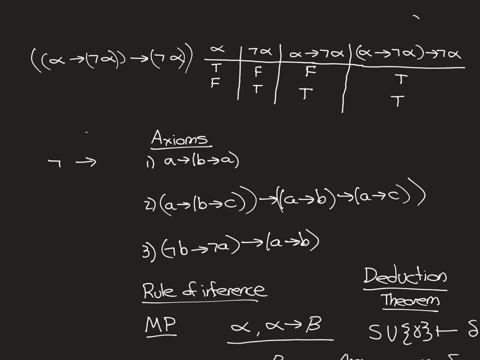 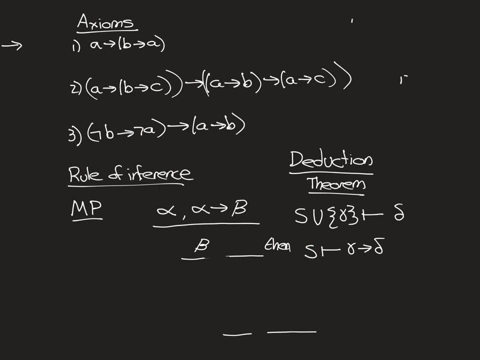 And then if we can prove our delta, which will be not alpha, from that premise and no other premises, just the axioms, then by the deduction theorem we'll be able to conclude that the empty set, ie no premises, 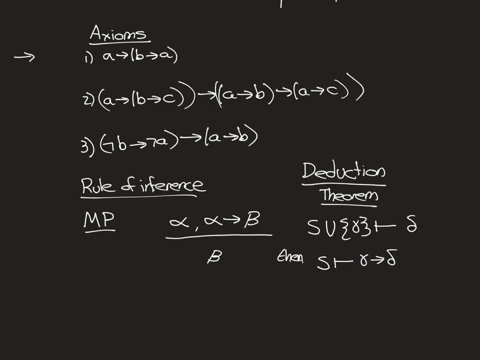 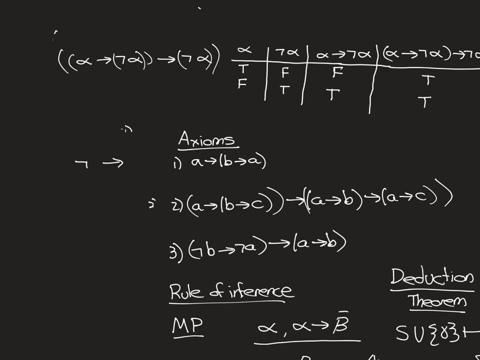 is able to prove. gamma implies delta, which is the statement that we've got here. This is our gamma and this is our delta. So that's how we're going to prove it with the deduction theorem. So let's finally, now that we've got the setup, begin. 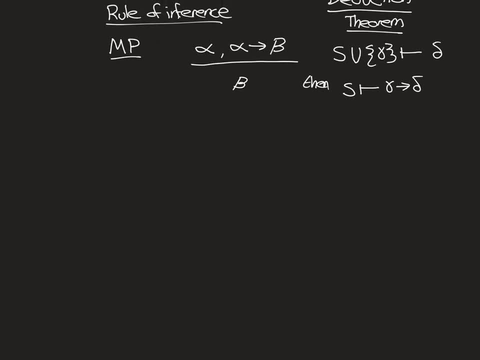 So, as I say, this is what I came up with. It is long and complicated. I really do apologise if there is a much simpler way of doing this. So, as I say, we're going to use the deduction theorem. So we're going to assume as a premise: 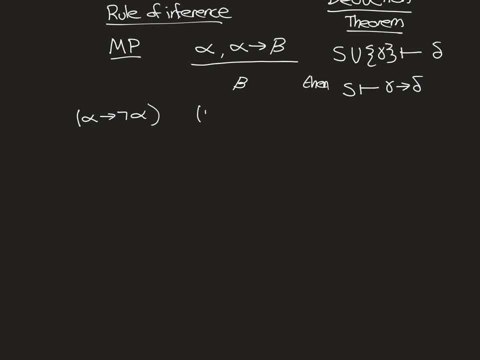 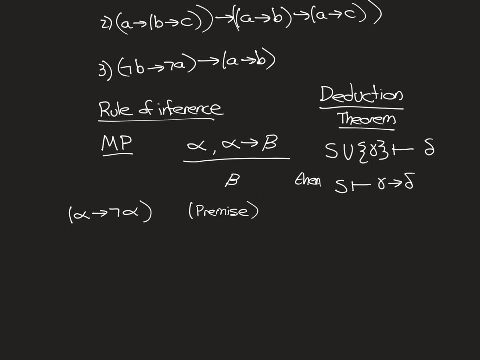 alpha implies not alpha, So I might put that as my first line in our proof. And now I'm going to have to think about what we're going to do next. So I think the next thing I'm going to do is I'm going to use axiom 3 here. 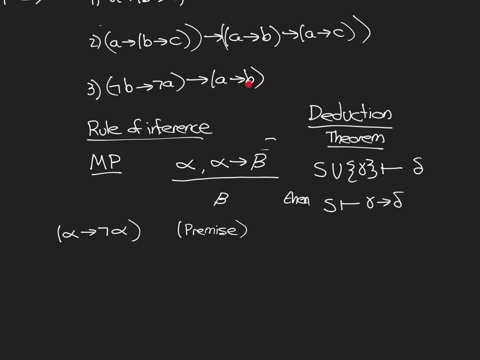 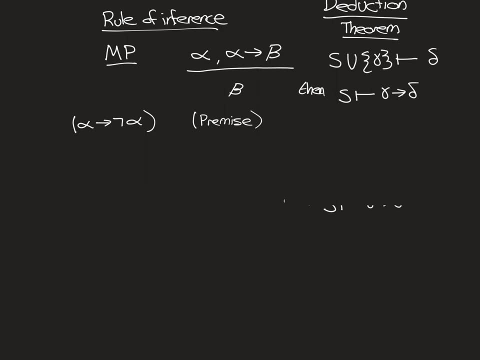 And I'm going to make my a alpha and my b not alpha. So then I have to put the not b up here, So it'll be not not alpha Actually. no, this is not what I want to do, Sorry. As I say, I did warn you this wouldn't be polished. 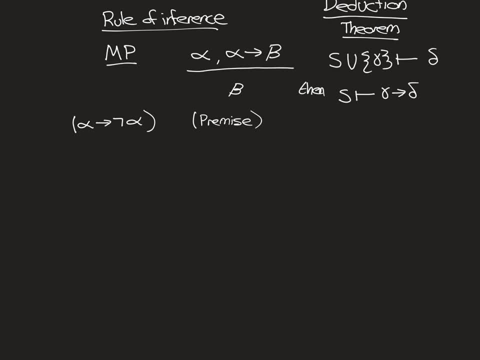 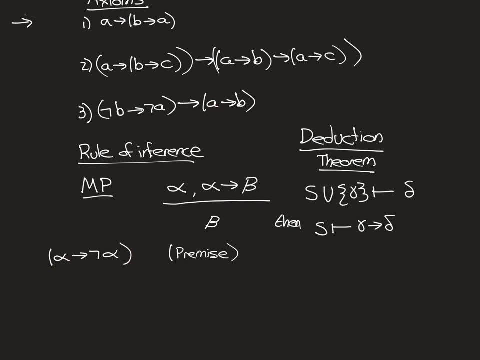 So what I actually want to get is: I want to get, I want to get a, I want to get this thing as my a and I want to get b as my- not alpha, Because if I was able to get this, then I would be able to apply modus pollens. 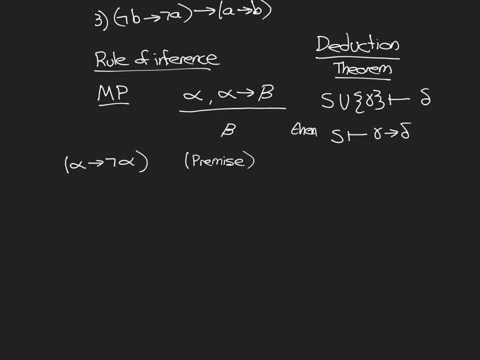 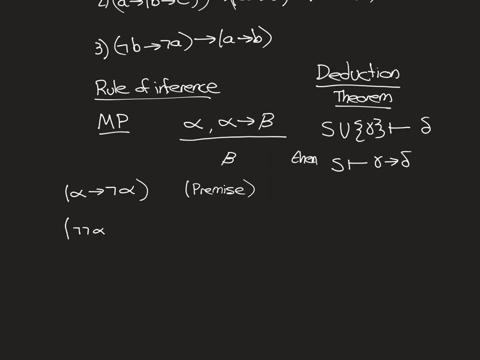 and get not alpha. So I'm going to fill that in. I'll keep it in view. So my b is going to be not alpha. So I was actually right. I do want not not alpha here. But then my a is not just alpha. 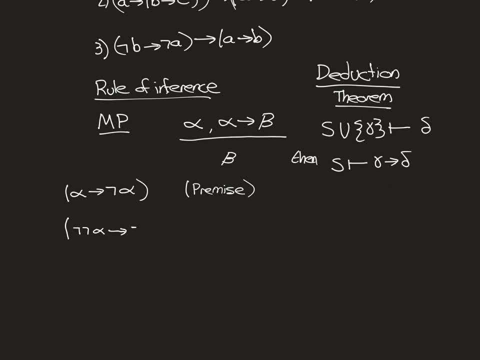 It's not. and then this whole thing here. So not whoops. alpha implies not alpha. And again note, alpha isn't necessarily a propositional variable. It might be a whole formula. It doesn't matter, Because even if it is a whole formula, 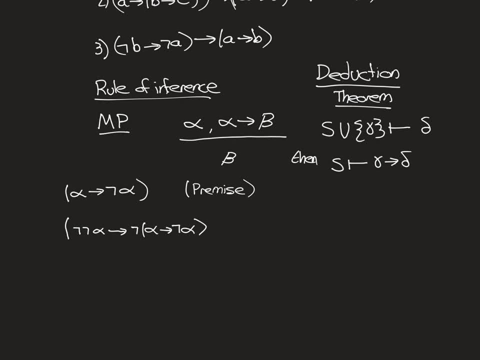 all of what I'm doing still applies, Whether it's a propositional variable or some whole formula. all of this argument is still going to apply because of the flexibility of these axiom schemes. So, as I say, the a here is this whole thing. 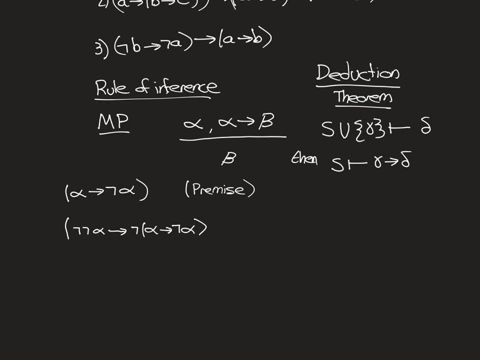 b is not alpha and a is alpha implies not alpha. So that's right. And then this will imply: a which is alpha implies not alpha implies b which is not alpha. So this is axiom 3, that we got that from. 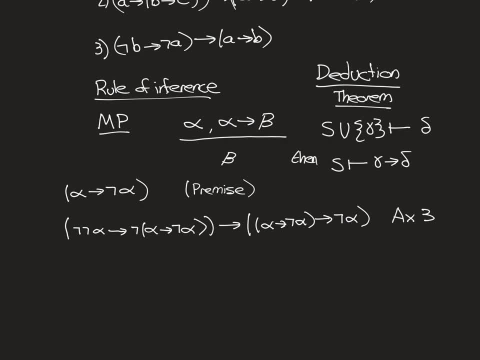 So I'm allowed that in my proof sequence. So so far I've had a premise. This is my first proof, This is my first line in my proof sequence And second, I've had axiom 3 as my second line. So the idea is that if I can get this thing now, 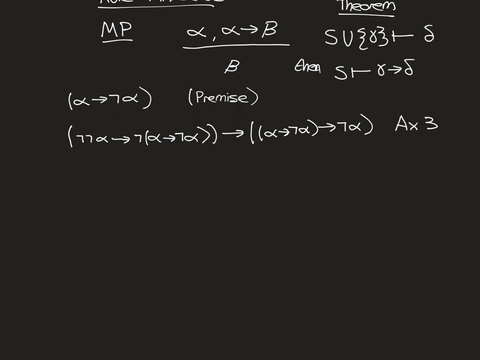 then I'll be able to apply modus pollens. So say, I had that, then I'd be able to apply modus pollens and I'd get this thing, And then I've got this, So I can then apply modus pollens with this and this. 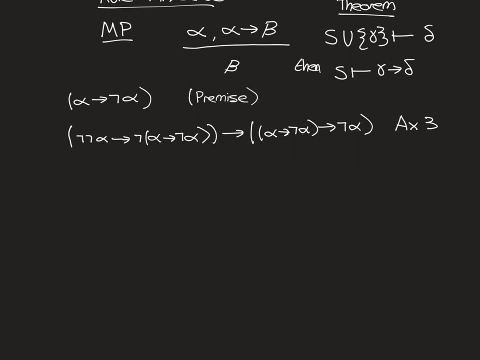 to get not alpha, And then by the deduction theorem I'd be able to conclude what we want: that no ax, no premises, just the axioms, is able to prove that alpha implies not alpha implies not alpha. So now my concentration is going on to getting this. 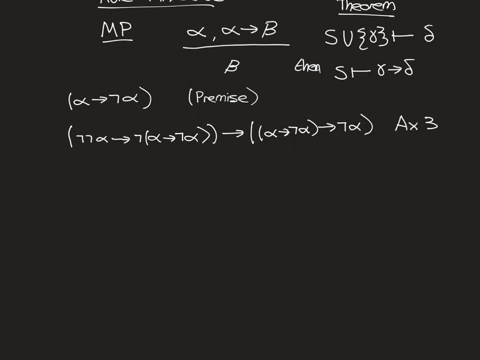 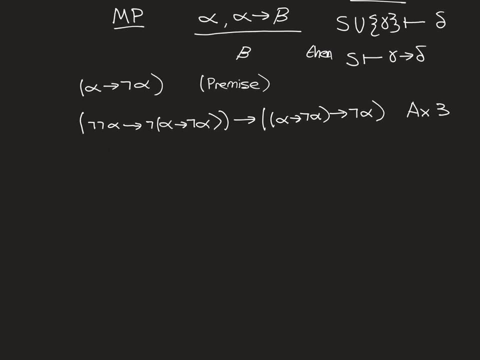 How do I get this? So, the thing that we're going to aim for- and there's going to be lots of sides to this proof, because we're going to need lots of other results, things that can be formally proved- So the way that I'm going to get this, 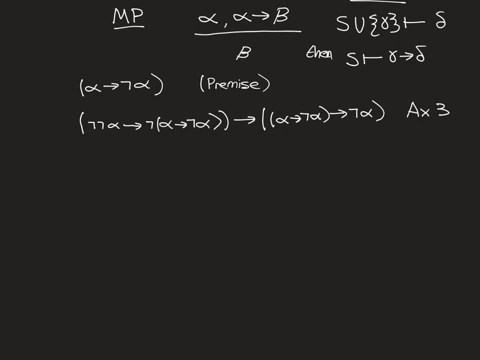 is: how am I going to get this? So we're going to write down axiom two next, And the axiom two that I'm going to have is not not alpha implies, not alpha implies, and I might have to correct this if we, if it goes slightly wrong. 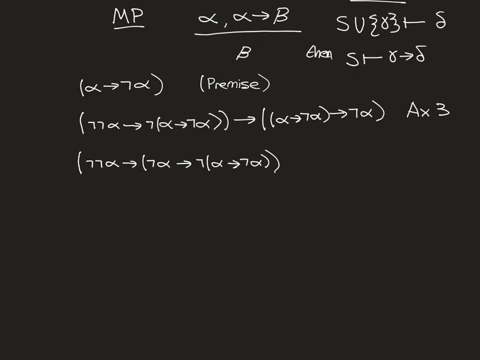 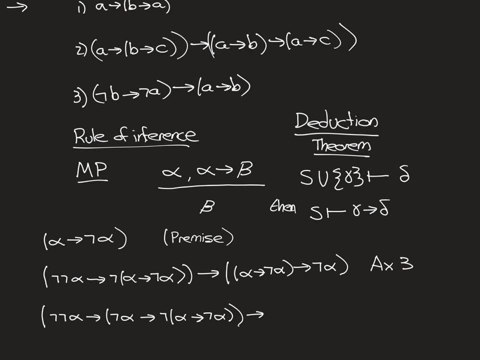 So alpha implies not alpha. This is what I think I remember doing, So let me clarify what I'm doing here. So we're using- so we're using- axiom two up here. This thing is a, not not alpha. is a, b is not alpha. 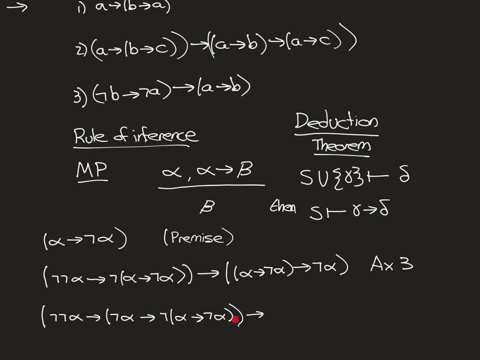 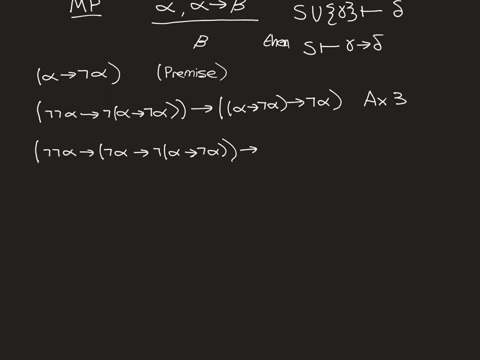 and c is not alpha implies not alpha. So all of that is c, And so I'm going to be able to put this here by axiom two. So splitting it up it goes to: not not alpha implies not alpha, And that's good. 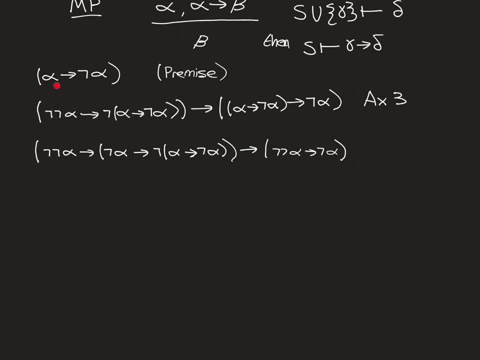 That's something we should easily be able to get From this. we'll need modus tollens, the right way round. So our axiom three isn't, strictly speaking, modus tollens, although I think you can be forgiven for calling it backwards, modus tollens. 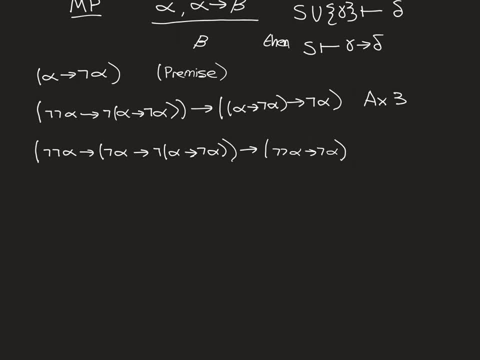 But we need to get modus tollens the right way round. ie a implies, b implies not, b implies not a, So that from this we will be able to conclude this, but we'll have to prove modus tollens. 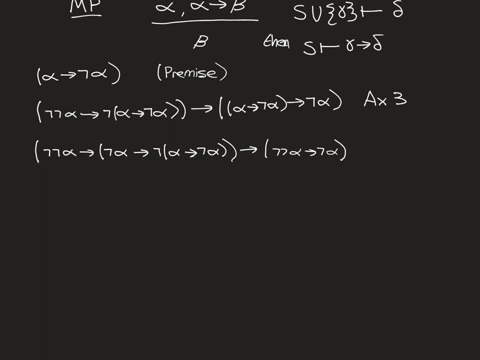 And that'll take a bit of work, But we should be able to get that from this premise And then we need to finish this. So this implies, and then it's this one implies this one. So not not. alpha implies not, alpha implies not alpha. 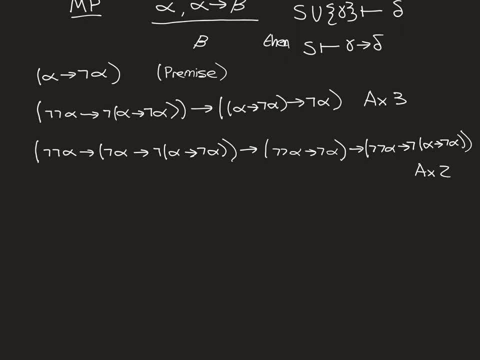 And that's axiom two there. And the use of this is that if I can now get this thing, then I'll get this here and there should be, for clarity, another set of brackets around that I'll get this thing. Then, if I can get this by modus pollens- 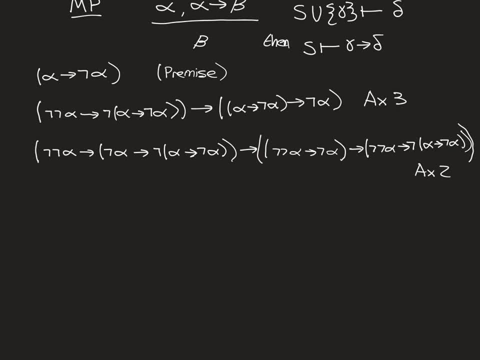 of course. then if I can get this thing, which I've already sort of said I'm going to be able to get, then by modus pollens I can get this, And oh, look, that is exactly what we want. 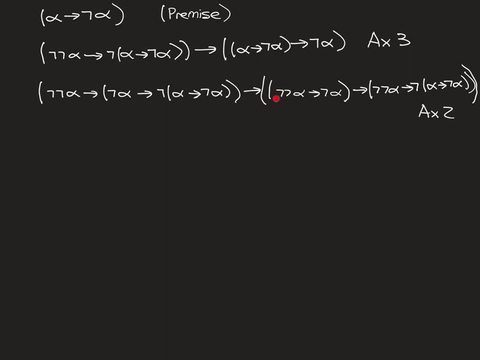 So what should we do next? I think, before I show you that we can get this, I should show you how we can get this. So this is actually beautiful. This is kind of a side proof, Or should I just put it in the main proof itself? 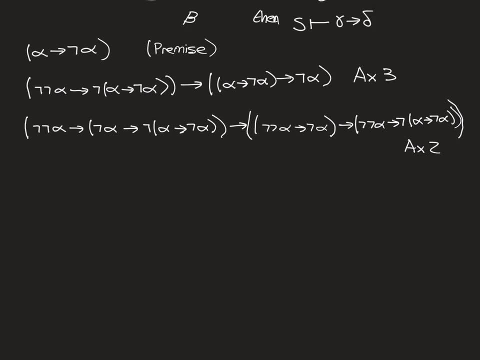 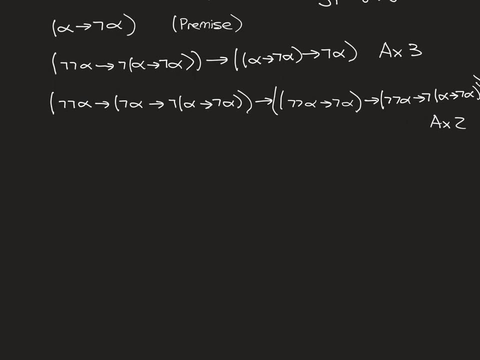 Maybe I will put it just in the main proof and make it all into one. I think that might actually be tidier. So how do we prove something like that? Well, you can prove anything. kind of A nice trick is that you can prove. 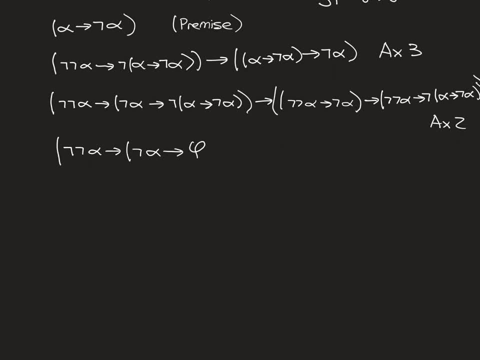 something actually of this form, Much more general. I can put in, you know, phi there, where phi is, any propositional formula you like, because what this says is that if not not alpha is true, then well, you know the moment that not not alpha is true. 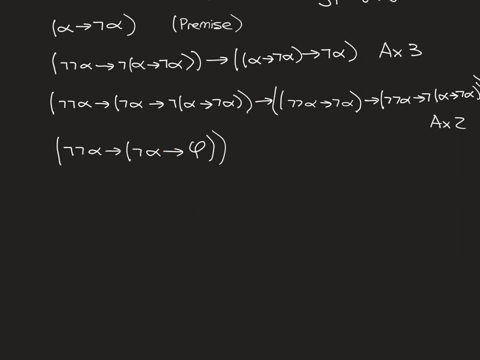 that not alpha is going to be false because this is not not alpha. So this one's going to be false and therefore it doesn't matter. This implication is immediately going to be true because it's going to be vacuously true, So it is going to be true. 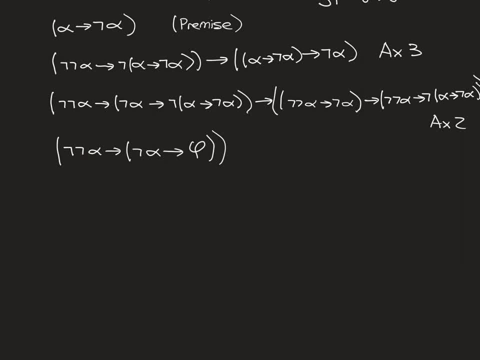 that when this one is true, this one is not, this one is true, And then when this one's false, then the whole implication is vacuously true anyway. So this is actually a tautology and something that we're going to be able to prove. 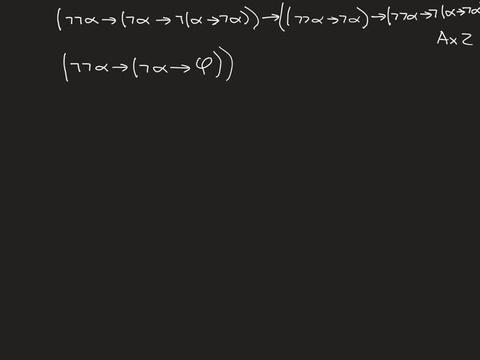 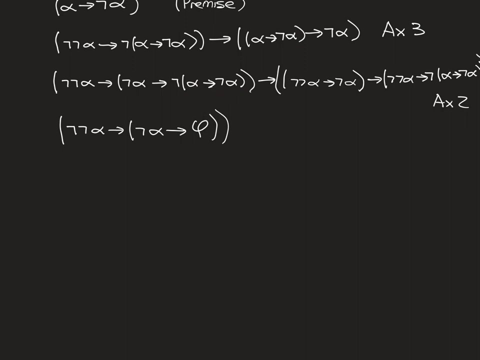 So how are we going to prove that? Let me remember how we prove this, So you can put whatever you like there and we will obviously stick in the thing that we want. which is not alpha implies not alpha, So we're going to. 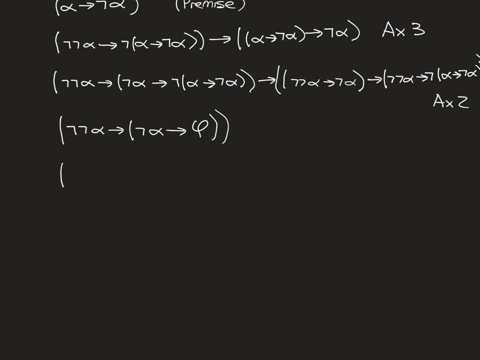 we're going to start with axiom one, I think, and we'll have, and then we're going to invert it with axiom three, So I'm going to put not phi in as my b, and then we're going to want not, not alpha. 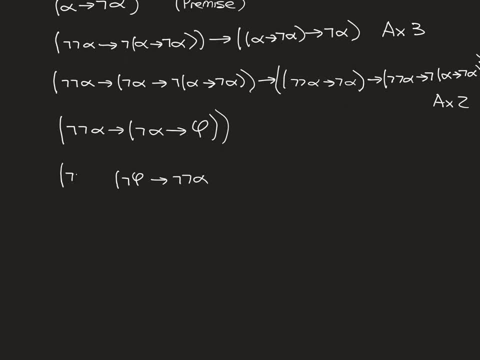 I think. So I think this is whoops. this is what we want, Not not alpha applies, And I will just rub this line out because we that's not part of the proof. In fact, I'm going to rub this line out as well. 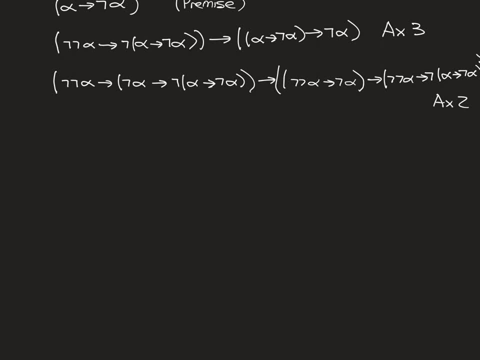 And we will put in our specific thing that we want, but be aware that you could have done this for a general phi. It doesn't have to be this thing specifically. So our next line of the proof is going to be using axiom one. 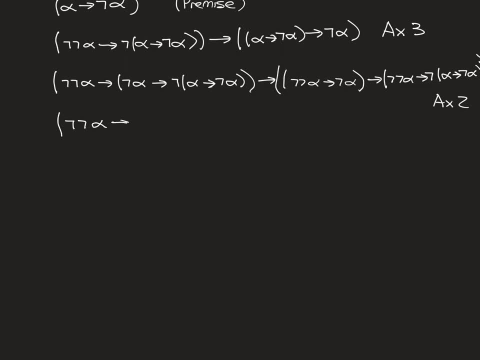 We're going to have as our a not not alpha, And then as our b we're going to have not, and then this whole thing. So we're going to have not not alpha implies not alpha- And then as our a. 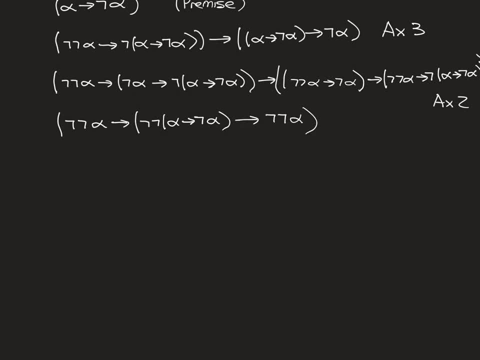 we have to have the same thing again. So it will be not not alpha. So does that have enough brackets in? I think that bracket's overkill there, So we'll get rid of this one. So this is, oh, and I put it on the other side. 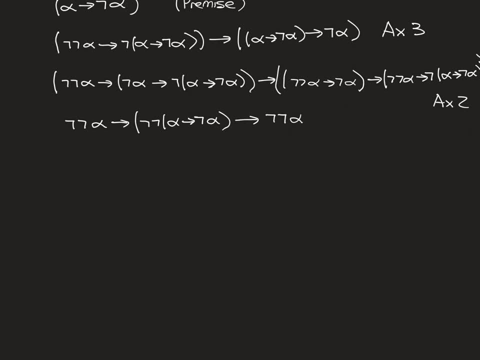 I shouldn't have bothered. Oh no, that one is important. Sorry, I'm getting confused, Apologies. So this is axiom one Here. Next, What are we going to do next? How are we going to conclude? not, not, alpha is the problem. 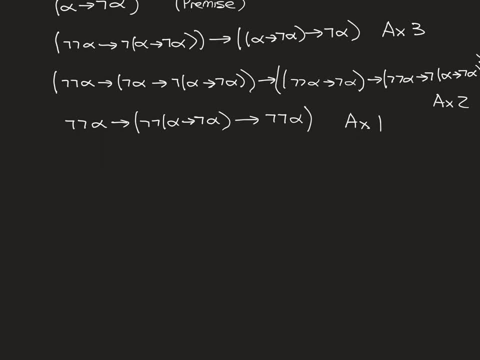 So we can definitely get that. Oh, this is why we should have done this as a separate proof. So we're going to have to use the deduction theorem. So apologies, Yeah, no, I can't do this all in one go. 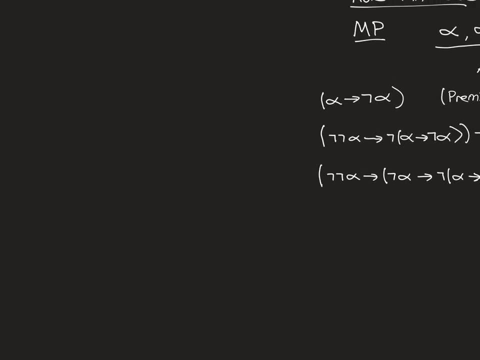 We're going to have to prove this side claim as a side claim. So my claim as a side claim- and we'll go back to phi- is that this is a something that is provable separately, And then we'll be able to just use it in our proof. 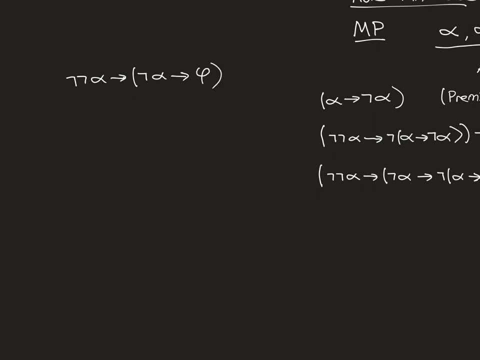 So not alpha implies phi, And this is what we want. where phi is going to be not alpha implies not alpha. So this is something that we're going to be able to prove, And the way we're going to prove it is by the deduction theorem. 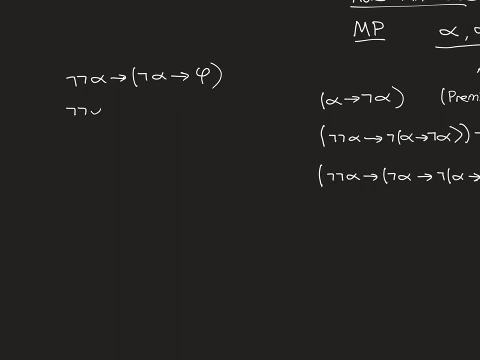 So we're going to take as our premise not, not alpha. We could try and prove it without the deduction theorem, but God knows how you do it. The deduction theorem helps hugely. So we're going to take not, not alpha as a premise. 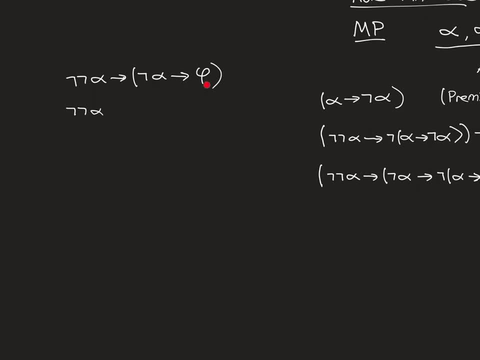 And then we're going to prove this part: not alpha implies phi, And then by the deduction theorem. then no premises proves is able to prove not. not alpha implies this thing. So we have as our premise not, not alpha. 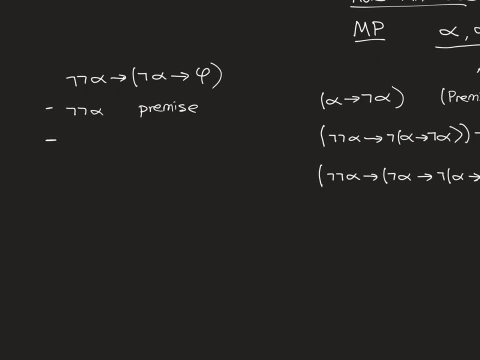 And then we're going to do what I said, which was use axiom one, So we'll have not- not alpha implies, and then we're going to have not phi as our b And then again as our a, not not a. 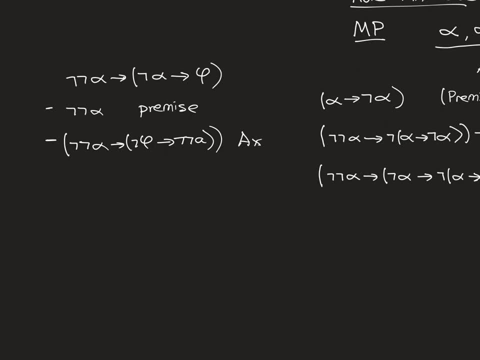 So that's axiom one. Then we're going to use modus ponens. So we have our premise here, we have this premise appearing in the antecedents of this implication here. So by modus ponens we then have not phi implies not not alpha. 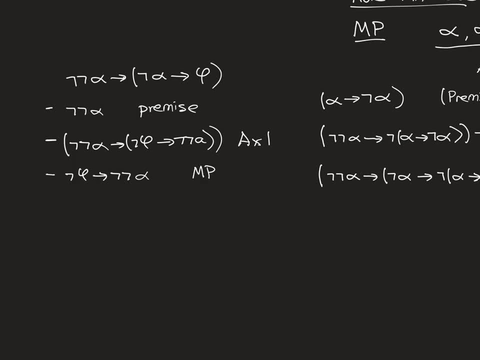 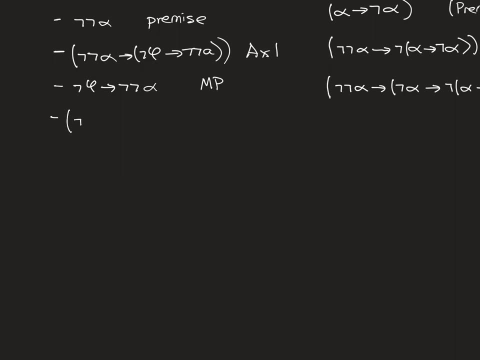 That's by modus ponens. And now we're going to use axiom three, So our b is going to be phi, so we'll have not b which is not phi. And our a is going to be not alpha, so we'll have not a which is not not alpha. 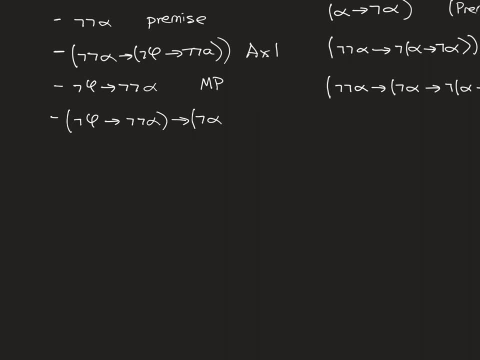 implies, and then a implies b, so not alpha implies phi, And so that's by axiom three, And then we'll apply modus ponens Here. we've got this, it's here in the antecedent here. So modus ponens with those two. 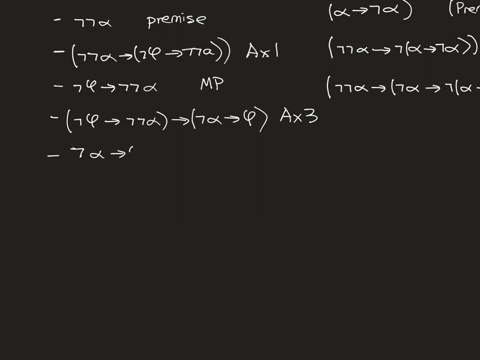 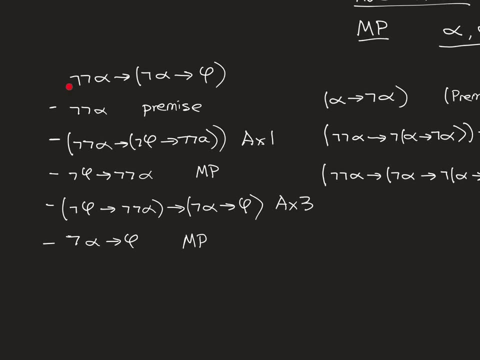 gives us then that not alpha implies phi, which is exactly what we wanted. So this is by modus ponens, And then by the deduction theorem. then we have what we wanted that not not alpha implies, not alpha implies phi. So this is always provable. 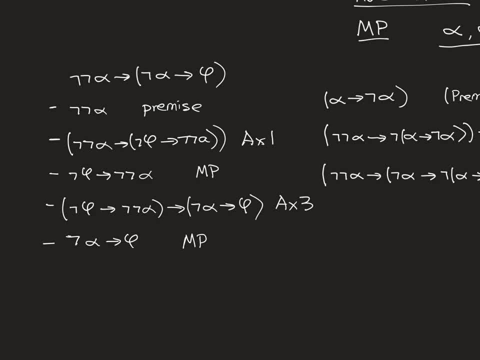 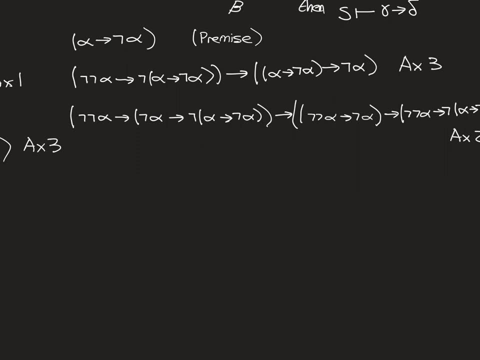 with no premises, just from the axioms. So what we're now going to do is use the fact that we know that thing is provable here. So we're going to just now stick in not not. alpha implies not alpha implies not alpha. 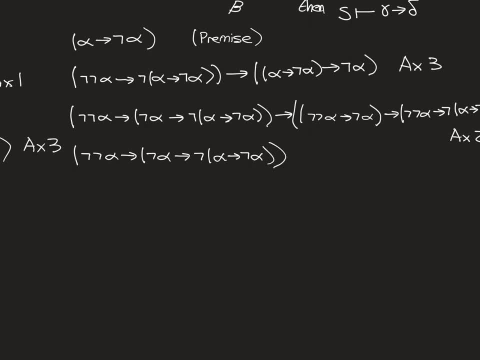 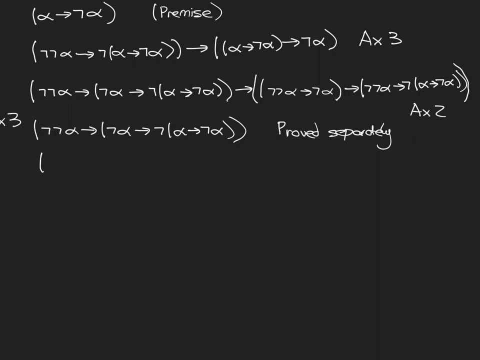 implies not alpha, which we've just proved separately, Separately. And now now we can apply modus ponens, because we've got the antecedent of this huge, great implication here, So we'll then get the consequence just left over. 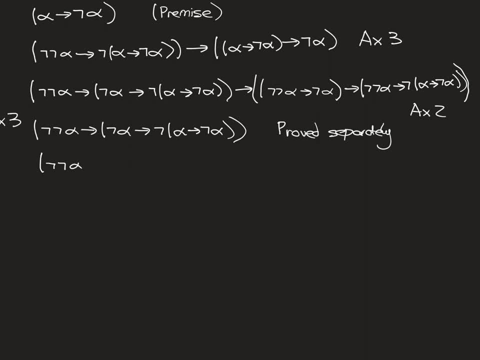 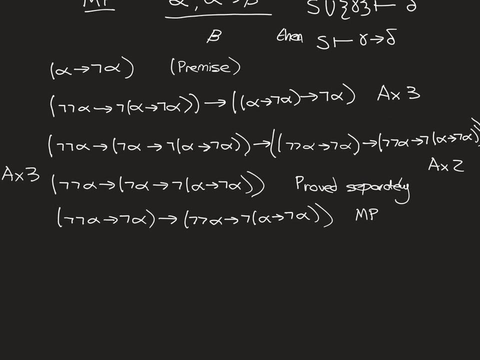 So we'll have not not. alpha implies not, alpha implies not, not alpha implies not, alpha implies not alpha. And that's by modus ponens. So we're getting closer, So, um, we are getting closer, much closer. So if we just 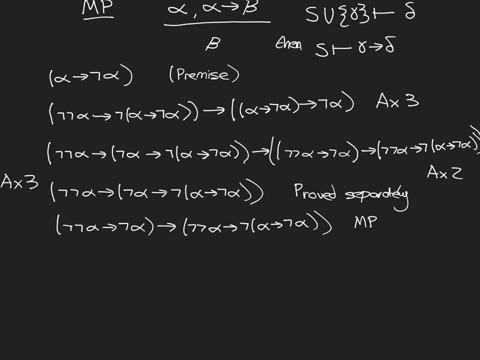 just take a step back and look at our overall strategy. So we've, if we get this thing now, we'll be able to apply modus ponens and get this thing, And then, by modus ponens, we will have this thing. 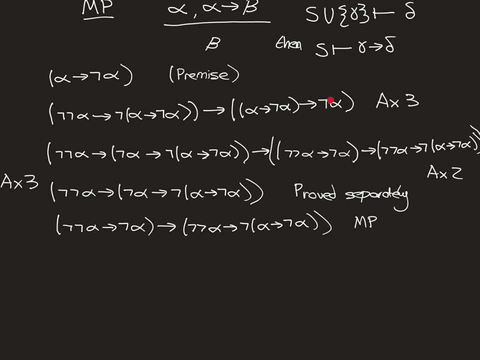 And then we can put this premise into here and get from modus ponens this thing, which then means we've got what we wanted. We're aiming for not alpha, remember? And then by the deduction theorem we're then going to conclude that 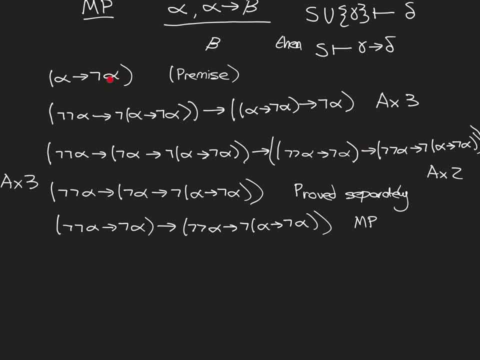 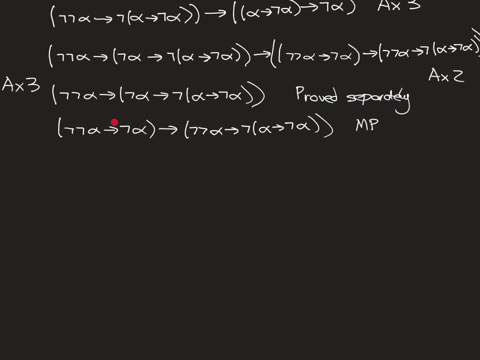 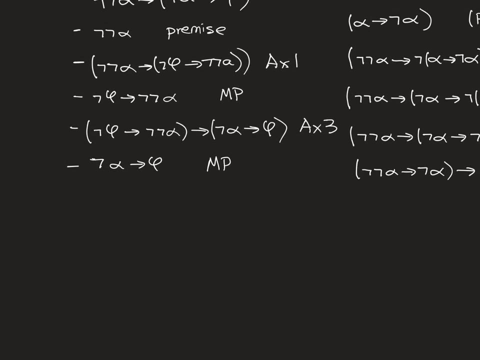 from no premises, we would have been able to conclude that alpha implies not, alpha implies not alpha. So next, I need to convince you that we can have this thing. So this is going to require me to prove modus tollens to you. So this is going to be a separate proof as well. 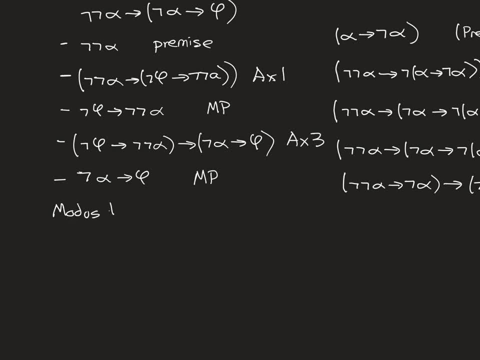 So modus tollens is not a rule of inference in our Hilbert system. Uh, it's some a rule that is going to be derivable in our Hilbert system as being true? Uh, but it's not. it's neither an answer. 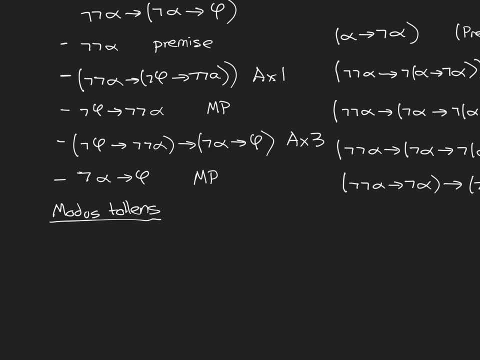 it's neither an axiom, nor is it a rule of inference or a rule of deduction. So it is that A implies B implies not, B implies not A. So a kind of axiom free. but the right way round is what's called modus tollens. 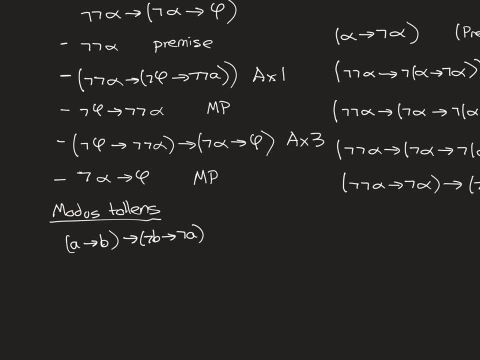 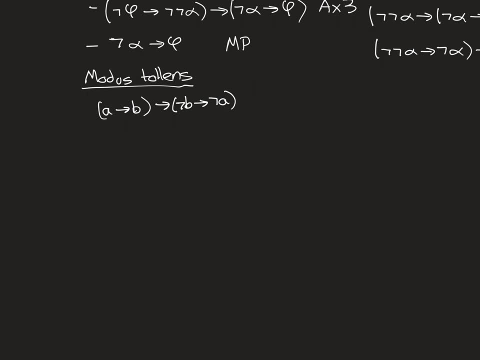 And this is always going to be a tautology and it's something that's provable in our Hilbert system. And again, A and B aren't necessarily propositional formulas. They could be. they're not necessarily variables, They could be complicated formulas. 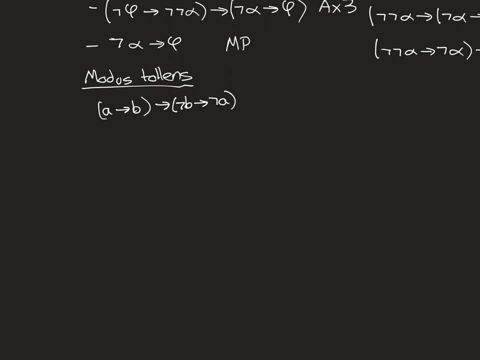 So how are we going to prove this? So I think, the way you prove, we're going to need quite a lot. to prove this, We're going to need double negation introduction, double negation elimination and um, hypothetical syllogism as well. 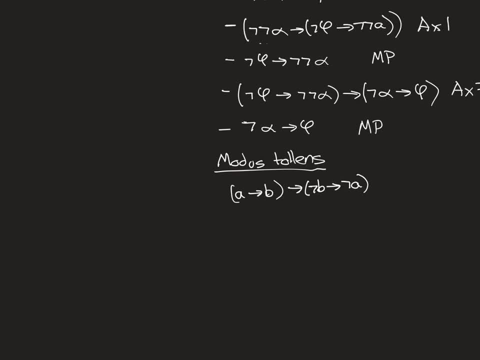 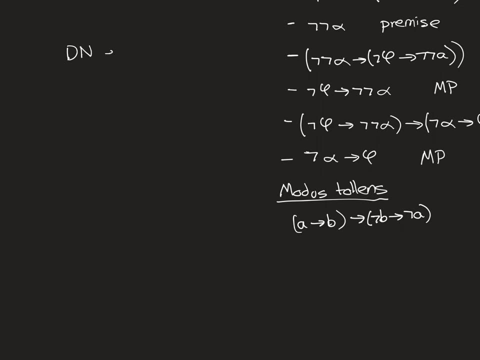 So we need other uh rules of logic that are derivable in our Hilbert system, provable in our Hilbert system. So let's start with derivative double negation elimination. So this is the name for the fact that something that is always provable 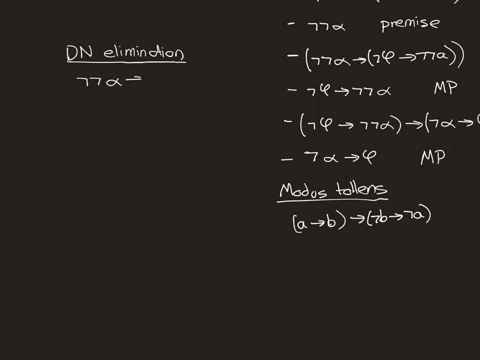 in our Hilbert system, is that not? not alpha implies alpha. So this is another statement like what I've got over here, this one about phi. Where is it? Um, where did I write it? So like this statement is always provable. 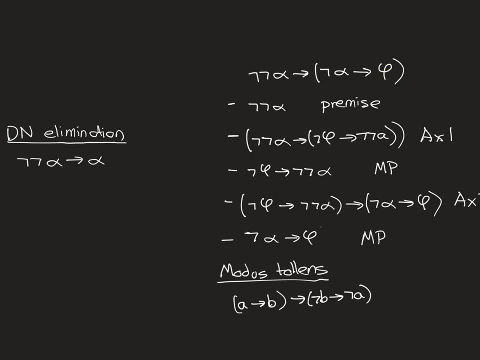 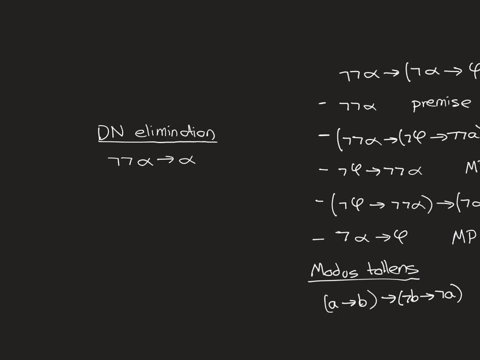 no matter what alpha and what phi in our Hilbert system, And this one, Moses-Tollins, is always going to be provable. This is another one that's always provable And it's named as well: It's called double negation. 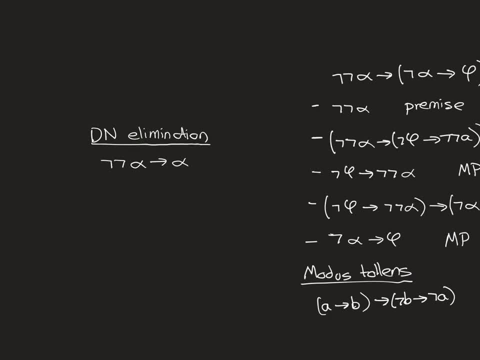 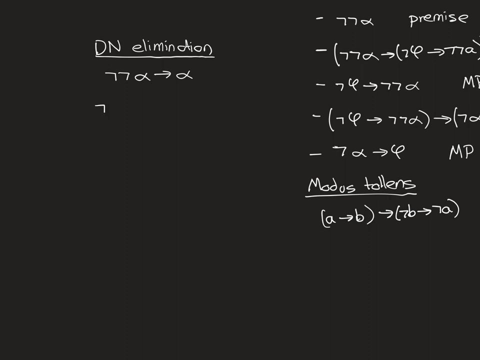 which I've abbreviated down to dn elimination. So how are we going to prove this? Probably by the deduction theorem as well. Everything is by the deduction theorem. It's so so much easier to prove things by the deduction theorem, So we'll take as our premise. 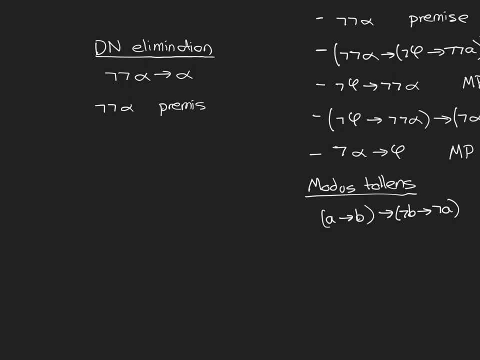 not, not alpha, And we're going to derive alpha And then by the deduction theorem we'll be able to conclude that, with no premises, not not alpha implies alpha would be provable. So how are we going to do this? Oh, how do you do this? 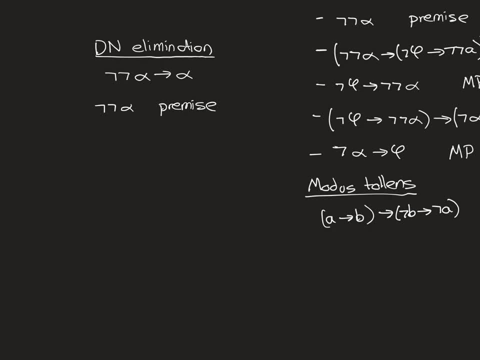 So not not alpha. We would then get. do I remember how to? I might have to pause this to remember how to prove this. Ah, yes, I've remembered now. So we firstly apply axiom one, So not not alpha, imply. oh, and I haven't told you. 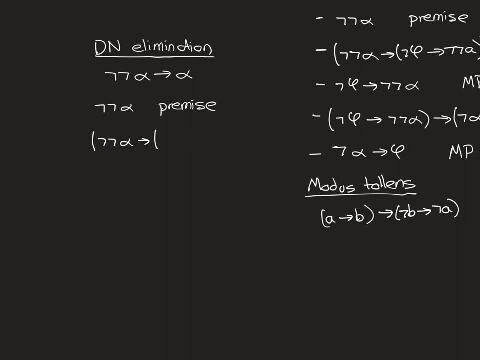 what we're doing with axiom one. So we're putting not, not alpha as a And then as b. I think we put not, not, not alpha as b, And then of course implies a, So not, not alpha. So that's by axiom one. 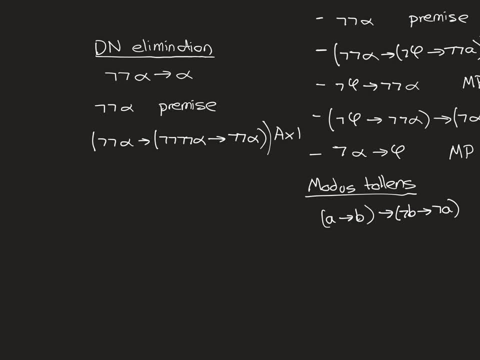 Another bracket there. And then modus ponens. We have our premise here. Here's the antecedent. So by modus ponens we then get that not, not, not alpha, for not implies not, not alpha. That's by modus ponens. 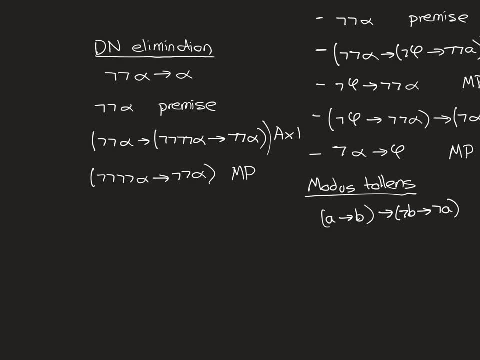 And now we're going to apply axiom three twice So, axiom three, with this thing that we've just derived in the antecedent, in the implication. So this will imply: so this bit here is our b and this bit here is our a. 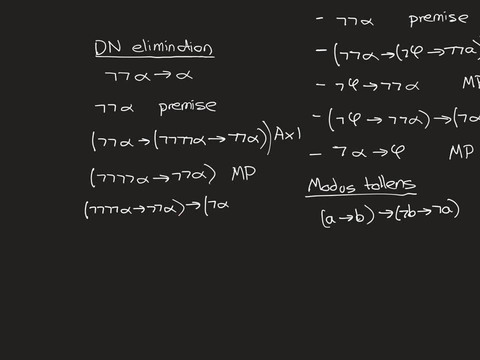 So a is going to become not alpha, or a is not alpha And b is not not, not alpha. So then we've got this Here. it is in the antecedent, So I should just write that that's by axiom three, So by modus ponens. 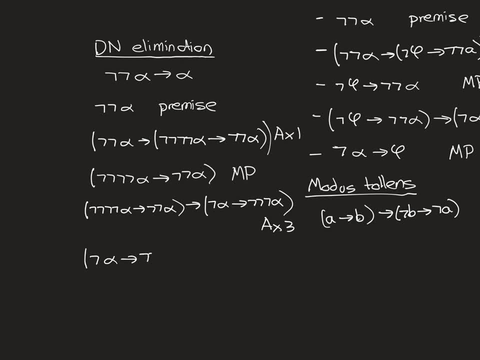 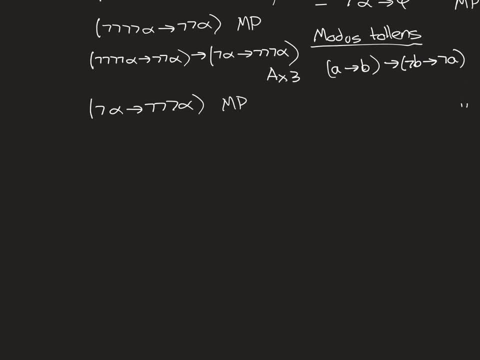 we then have that not alpha implies not, not, not alpha. And now we're just going to apply axiom three again. So not alpha implies not, not, not alpha. It's true by axiom scheme three that this implies not. not alpha implies alpha. So that's again axiom three. 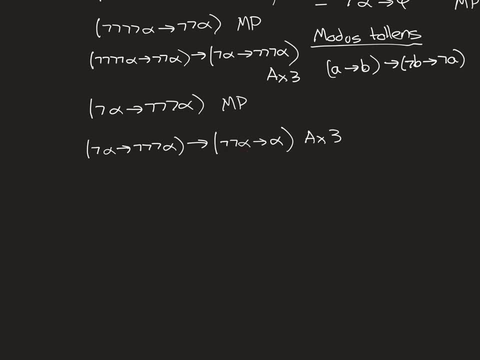 where this time a is not not alpha And b is alpha, And then we've got not b and not alpha, not a here Modus ponens again, because this obviously is the same as this. So we'll then get not. not alpha implies alpha. 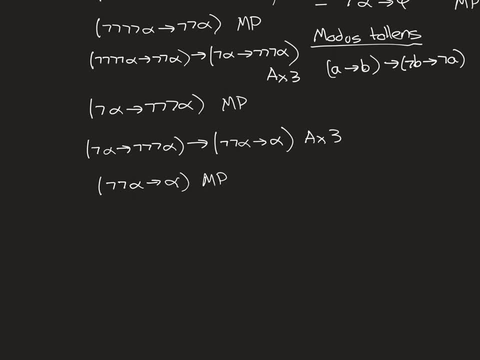 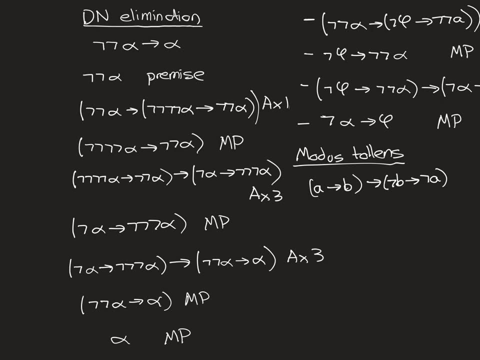 And excellent. We have not not alpha as a premise. So again, by modus ponens, we then get alpha, And hence then, by the deduction theorem, we're able to conclude that from just axioms we would be able to. 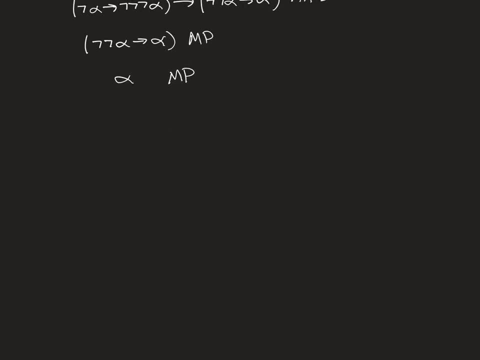 get not. not alpha implies alpha. So that's how you prove double negation elimination in this Hilbert system. Now double negation introduction, which is the opposite thing. It's that it's always true that alpha implies not, not alpha. And this one, I believe you just. 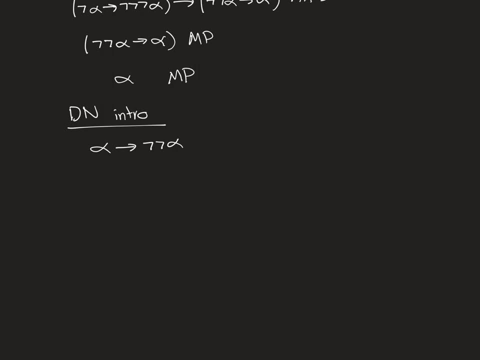 apply double negation elimination and then apply axiom three. So we're going to use double negation elimination on not alpha. So we're going to have not not. not alpha implies not alpha. So you see, I'm just using here double negation elimination. 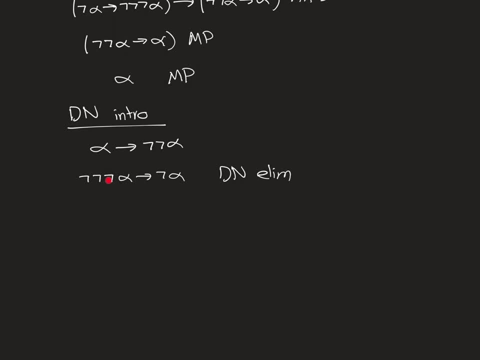 But instead of putting in alpha to double negation elimination- and having not not alpha implies alpha- I've put not alpha in And double negation elimination is true no matter what alpha you put there, So I can put in particular, not alpha. So this is true. 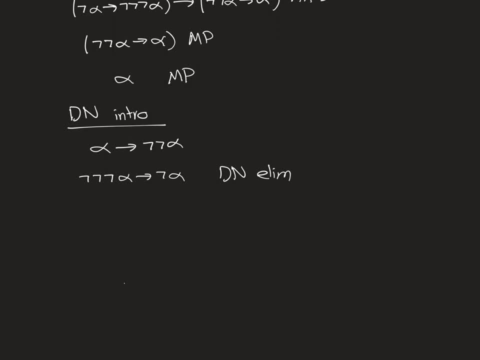 So this is true by double negation, elimination, And now I think I can just use axiom three to fix this. So this is one that we don't actually need the deduction theorem for. So by axiom three, not, not, not alpha implies not alpha. 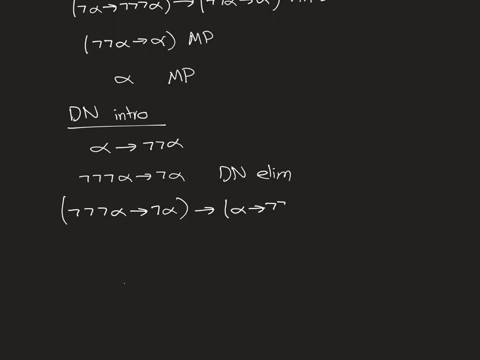 implies alpha, implies not, not alpha. That's something of the form axiom three. And then, of course, modus pollens. now to get alpha implies, not, not alpha, And then I'm done. That's what I wanted, I've proven this. So there's double negation. introduction. 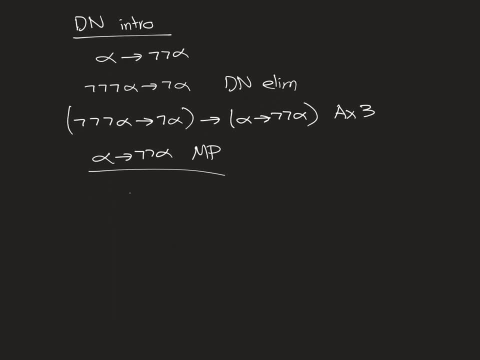 So those are two nice rules of logic that are provable in this Hilbert system- Double negation elimination and double negation introduction- And I'm going to need them. The reason I'm bothering with this is I'm going to need them to prove modus pollens. 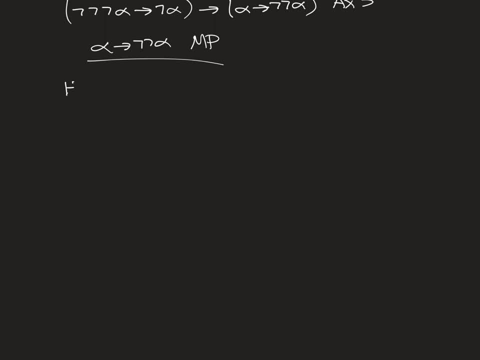 Right. The final thing I'm going to need for modus pollens is something called Hs, Which has a fancy name. It's hypothetical. Am I spelling this correctly? Hypothetical syllogism, Syllogism. Apologies if that's spelt wrongly. 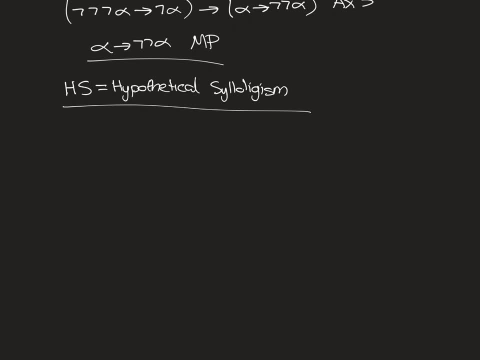 So this is a really complicated name for something that's really simple. It is that if you have the two premises, So my set of premises is going to contain that it is true that alpha implies b. Sorry, a implies b and b implies c. 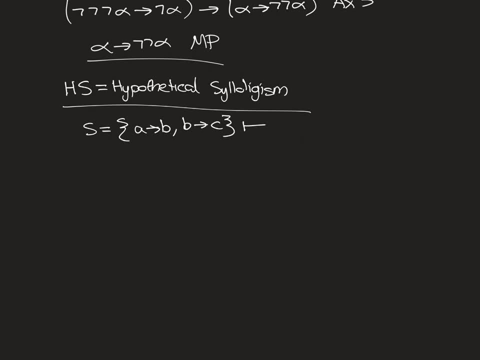 Then from that it is provable that a implies c And this the proof. So this is obviously really common sense. You know, if it's true that a being true implies that b is true And if it's true that b is. 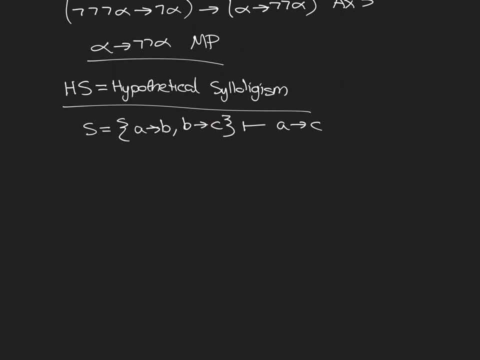 when b is true, it implies that c is true, Then it is true that the implication that a being true implies that c is true is also true. And the way that we would formally prove it is again by the deduction theorem. Let me just remember how we do this. 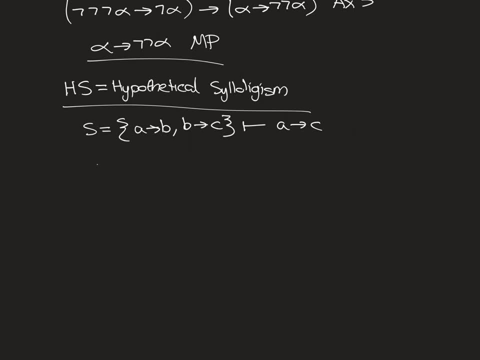 by the deduction theorem. Oh, yes, I remember, Or at least I think I do. Yes, So we would take our set as specified with these two things, These two premises in, And we'd add in another premise which is a. 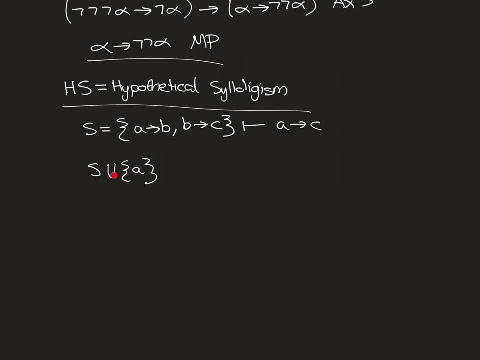 And then if we can prove from this c. So if this proves c, then by the deduction, theorem s alone would prove a implies c. But doing this is really easy, you know. So we've got a as a premise, We've got a. 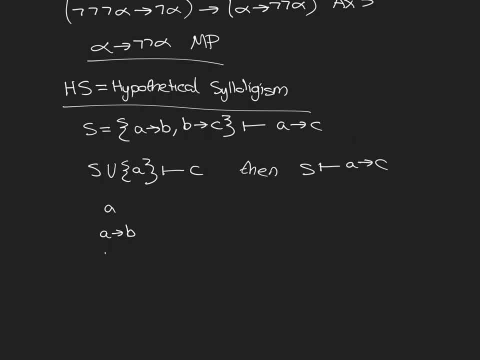 Sorry. yes, we have got a as a premise. We've got a implies b as a premise. So by modus ponens, we then have b. But we then also have b implies c as a premise. So by modus ponens, we have c. 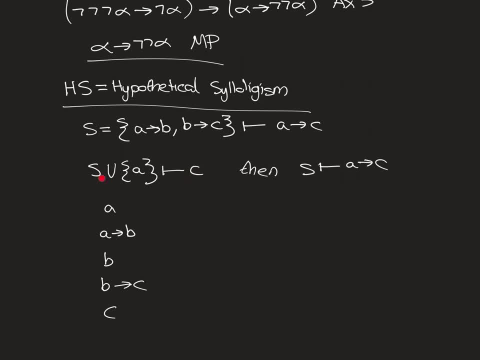 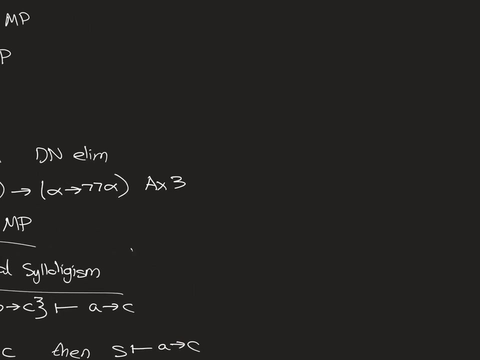 So we've derived, we've proven c from this set of premises. So by the deduction theorem from just s we would be able to prove a implies c. So that's how you prove hypothetical syllogism. And now I think we can prove finally modus tollens. 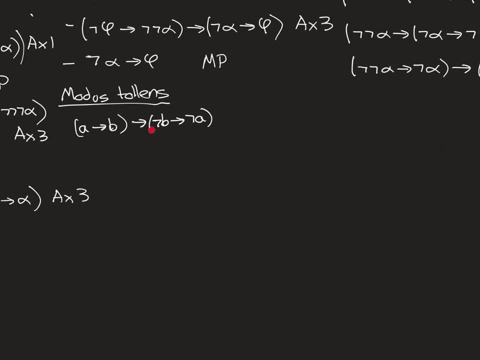 which is up here. So we want to prove this. How do we do this? How do we do this? So we do it by double negation elimination, double negation introduction and modus, and axiom three and hypothetical syllogism. 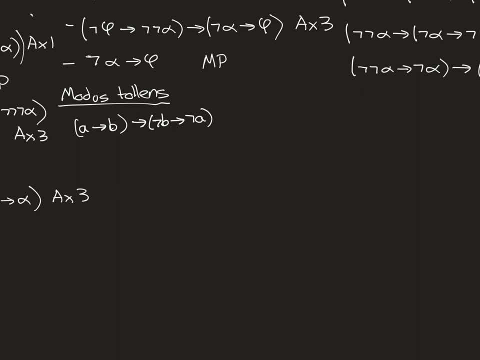 So how do we do this? We again- I'll have a pause just to think about this. So I think by the deduction theorem is again a good idea. So we'll take as our one premise a implies b And I'll stop writing out premise and axiom three. 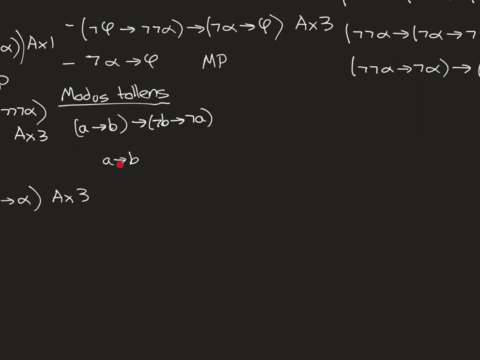 It takes too much time. So we'll take this as our one premise And then, if we can derive this thing, then by the deduction theorem this will be true. So we have a implies b, And then by axiom three. I think it's probably going to be a good idea. 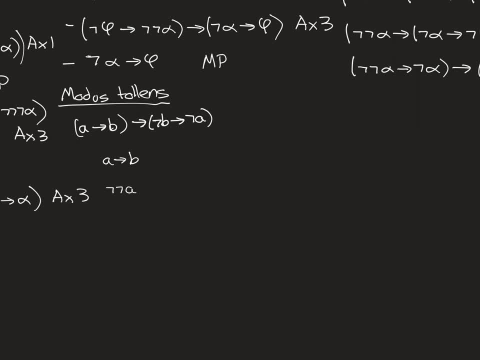 So we'll want not, not a implies not, not b implies. And then I think by axiom three, that is then not b implies, not a. And this is confusing because of course my b is now in the original way that I wrote my axiom scheme three. 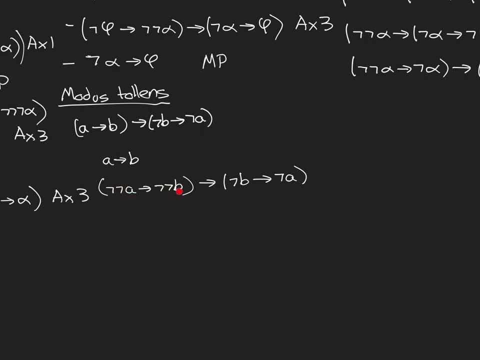 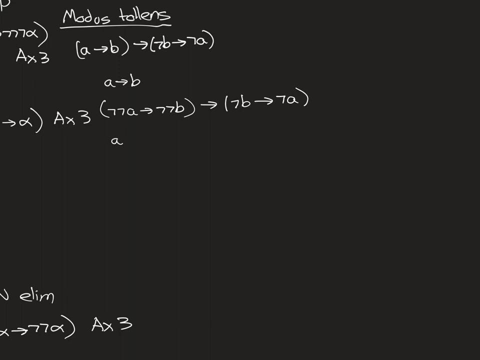 which is now not a And my a is not b. But I think then that all fits out. So that's axiom three. So I can have that in my proof. Then I'm going to have that. No, not this actually. 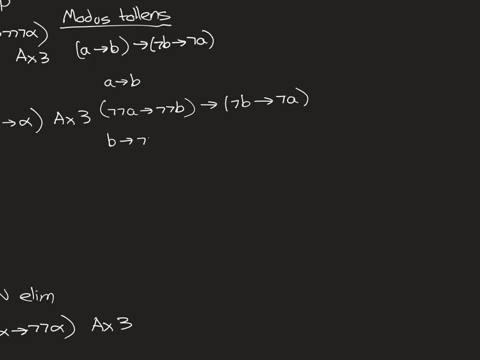 I'm going to have b implies, not not b, which I can have because I've proven double negation introduction in my Hilbert system. So I can have that in my proof because I've now proven that separately, Then by hypothetical syllogism. now 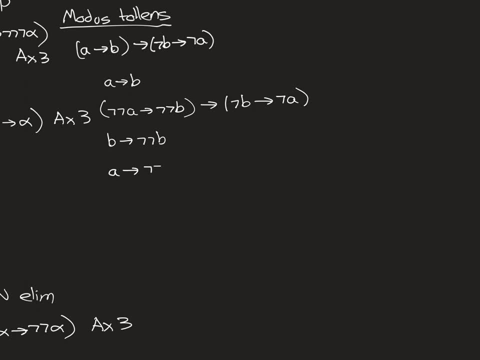 I know that a implies not not b, And I also know by double negation, elimination that not not a implies a. So again by hypothetical syllogism, I should have said here: you know, I'm applying hypothetical syllogism on these two that I've got here. 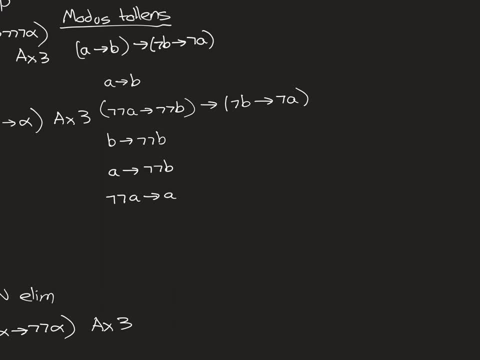 And I've already proven that this is an acceptable, provable law of logic that holds true in my Hilbert system of proof, Which is why I'm accepting this argument. So because a implies b and b implies not, not b, I've then concluded that a implies not, not b. 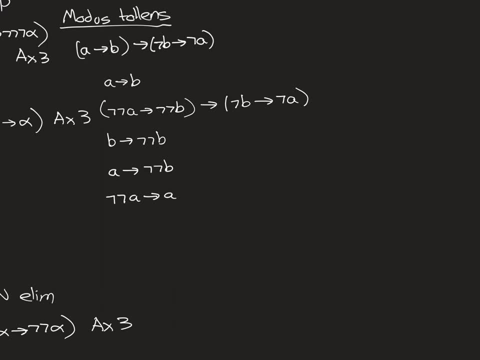 And similarly here I'm going to use hypothetical syllogism on this one and this one. So because not not a implies a and then a implies not not b, I'm going to conclude then that not not a implies not not b. 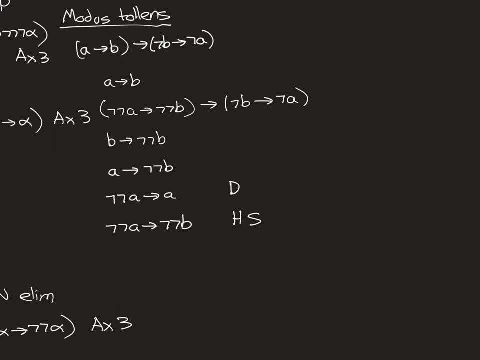 That's by hypothetical syllogism. This is by double negation elimination. This is by double negation introduction. Oh no, that's not by double negation introduction, That's by hypothetical syllogism again, And you get the idea. 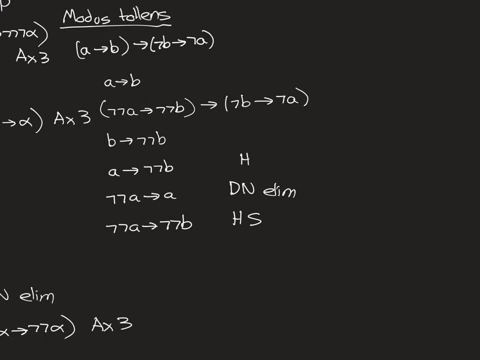 I won't write more of that out. So now I've got this thing here, which is my antecedent. So then, modus pollens- I get not b implies not a, which is what I wanted. So now I've got this thing here. 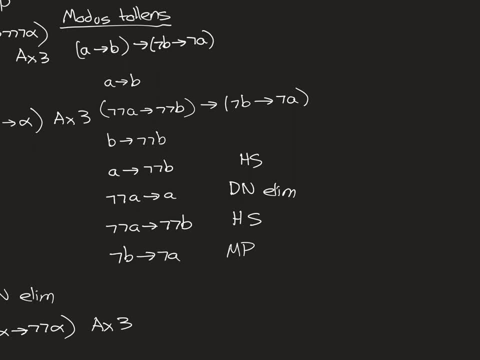 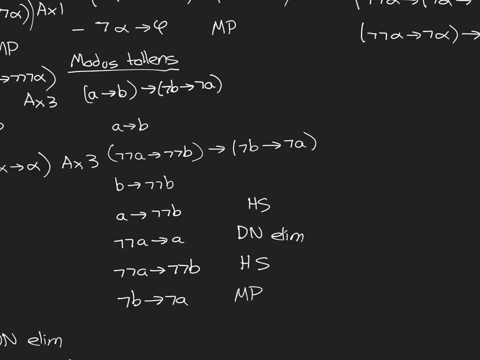 which is my antecedent. So then, modus pollens. so now, by the deduction theorem, it's true. This thing is true with no premises. So again, I've proven modus pollens Right. So all of that was to prove modus pollens. 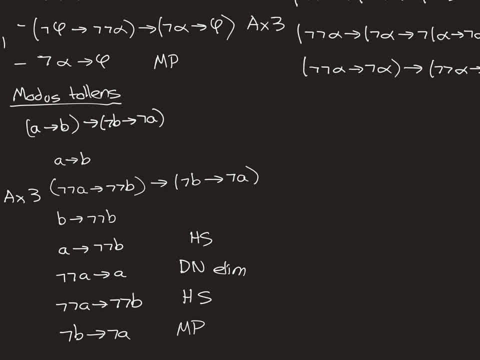 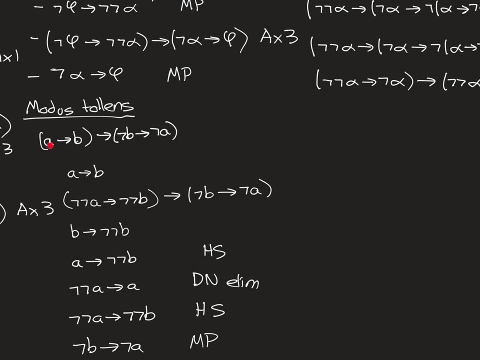 And the reason I wanted to prove modus pollens is now to plug in. for a, what am I going to have? I'm going to have alpha, And for b, I'm going to have not alpha, And then my not b is then going to be not, not alpha. 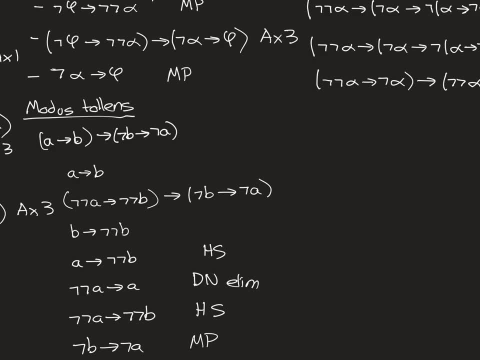 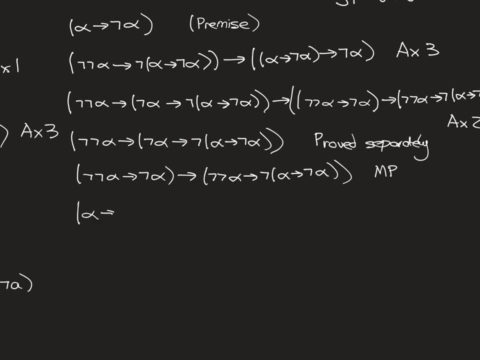 And my not a is going to be just not alpha. So going back up to our proof here, So by modus pollens, then alpha implies not, alpha implies not not. alpha implies not alpha. That's by modus pollens, mt. 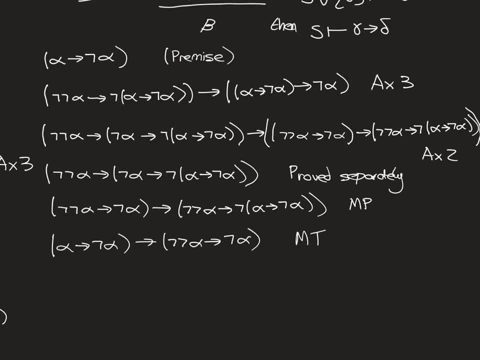 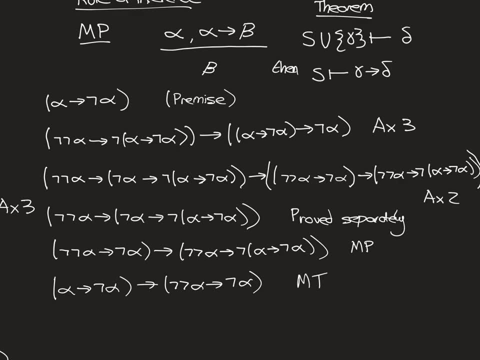 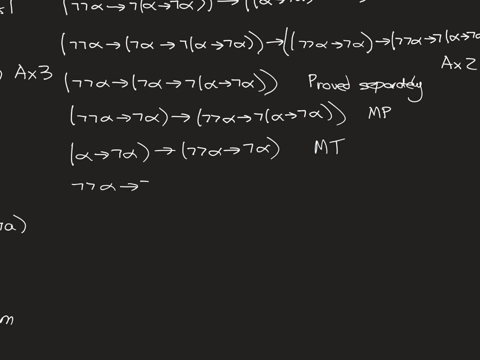 Now, because if you remember this bigger proof that we were trying to do here, we had alpha implies, not alpha as a premise. So I can do modus pollens now on this thing and therefore get not- not alpha implies not alpha. That's by modus pollens. 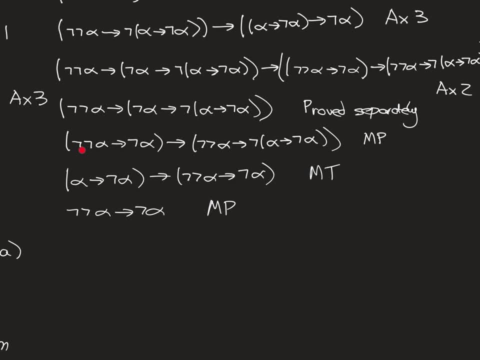 And now, where are we? Now I'm going to do modus pollens again, because I've got this thing, which is what I wanted for here. So now that means- and I think we're nearly there now, now that I've got not, not alpha. 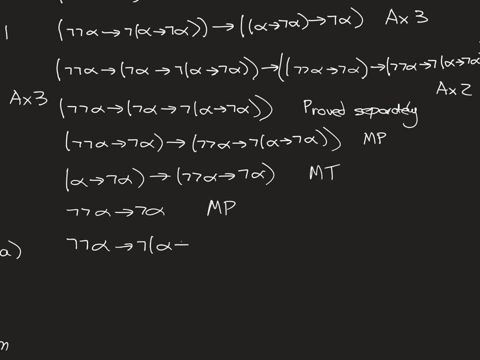 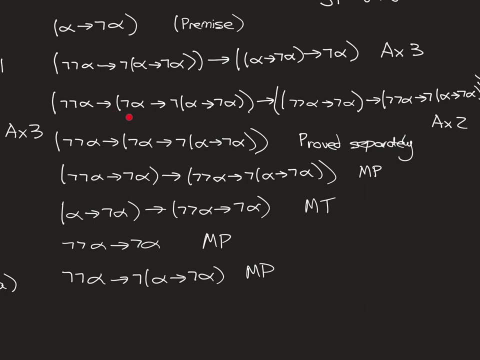 implies not alpha, implies not alpha. So again, that's by modus pollens. And then where do we go next? This thing I must stick in somewhere Over here. this is what I wanted. No, this isn't what I wanted here. 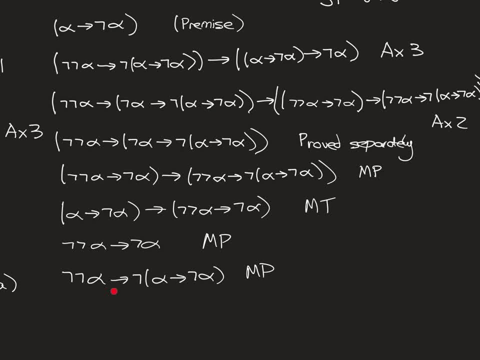 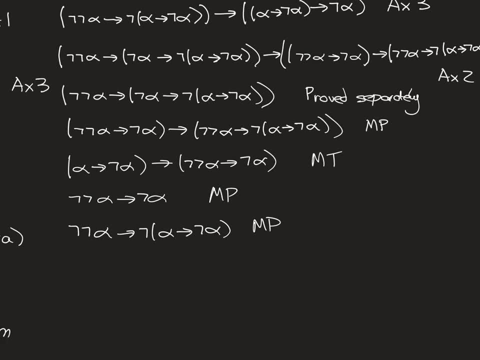 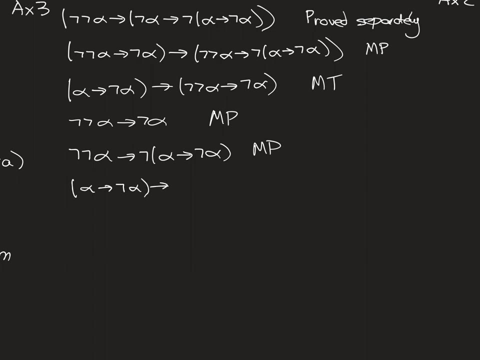 This is what I wanted up here. So here is this thing. So by modus pollens of this, with this, I'll then get this. So we then get alpha implies, not alpha implies, not alpha by modus pollens. And you might think: 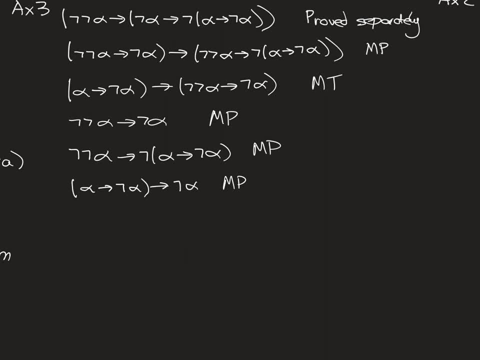 oh, that's what we wanted to prove. Are we done? No, Because, remember, we had a premise. in order to do all of our arguments, We needed that premise. So we now do have to finish the deduction theorem. So by modus pollens now. 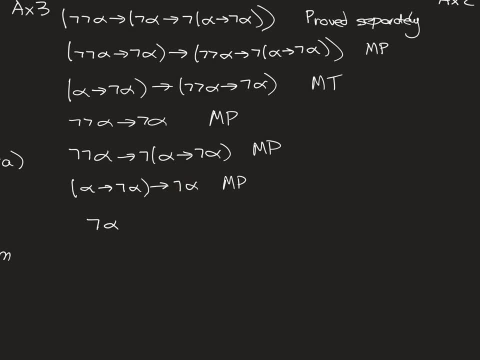 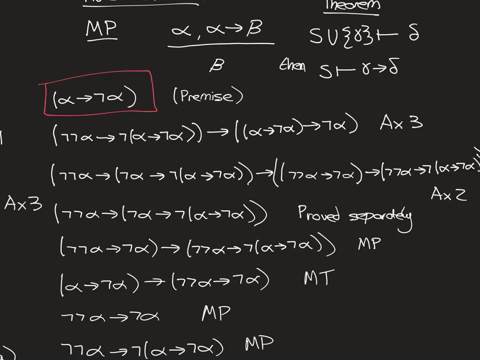 because this is our premise, we get not alpha, And hence with this one premise here- alpha implies not alpha- we were able to derive not alpha, And then by the deduction theorem we are therefore able to conclude that with no premises 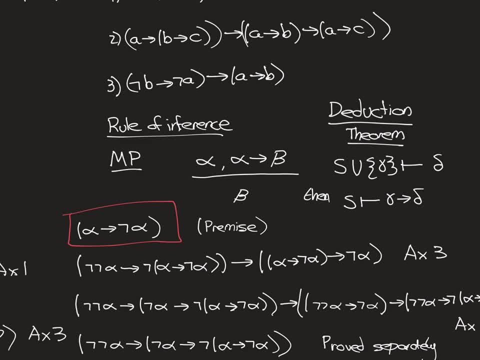 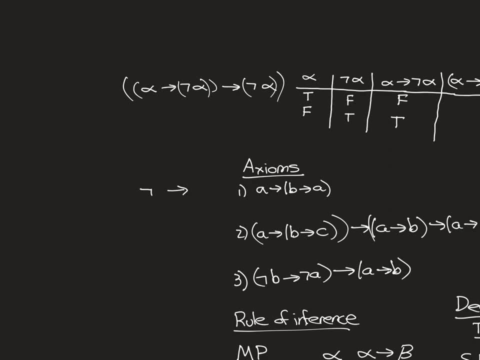 alpha implies not alpha implies not alpha. So this thing is provable within this proof system And we will finish there. As I say, it's a long explanation And it's made much longer because I did go to the trouble of proving all of the rules of the system. 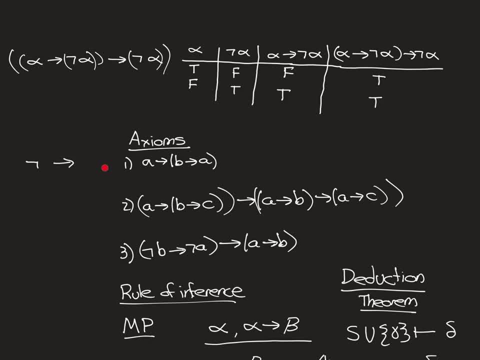 All of the rules of logic that hold true in this proof system that we needed to use in our proof. So I proved double negation introduction, double negation elimination, hypothetical syllogism and modus pollens. And I also proved another really nice result. 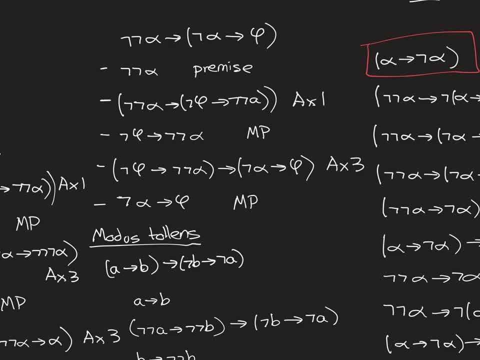 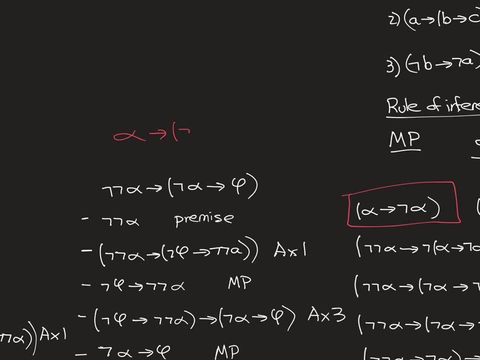 which is this one. This is really useful. I mean, this isn't the form you would normally see it in, The sort of more common form to see it in would be: alpha implies that, not alpha implies anything. You know we needed it in this form. 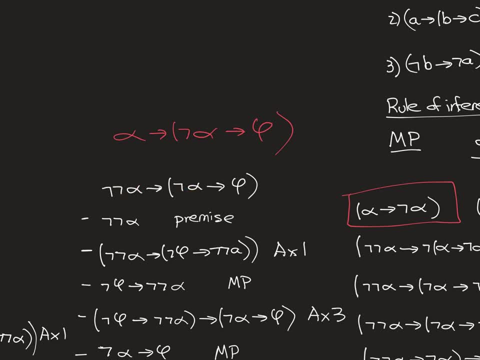 where we had the not not alpha here and the not alpha here, But this would be the more common form because obviously, when this one's true, this one will be false And therefore it's true that it implies anything. The same thing holds true here. 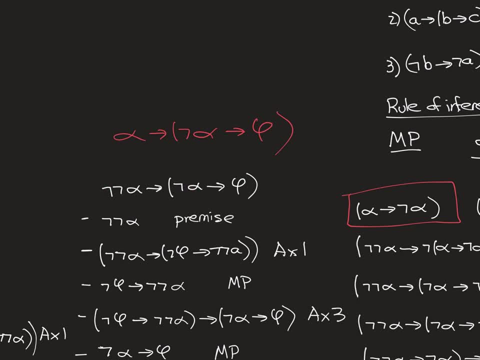 It's just slightly more complicated because of the additional not symbols, But you know the fact that all you need is a differing number of not symbols in between the two. So here there's a different number, Here there was a different number and it works. 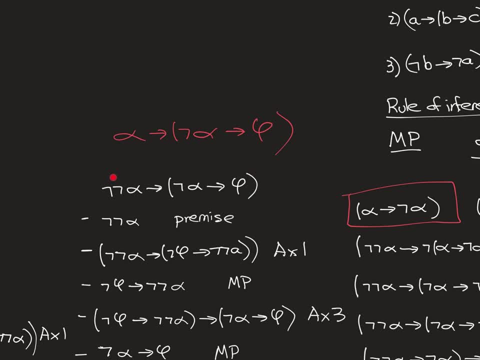 It's something very handy. I think some people do have a name for this. However, I don't think it's consistent people using the name for this, So I don't remember the name for this, but it is a really useful rule of logic. 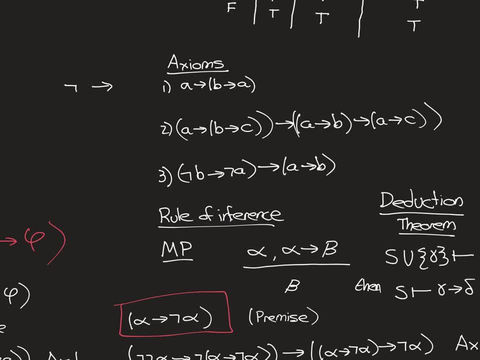 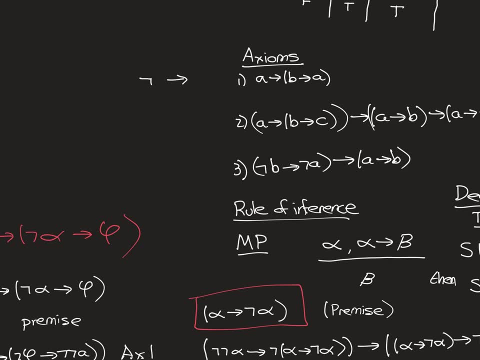 that holds true in certainly this Hilbert system, or is provable in this Hilbert system. It's always a tautology in propositional logic, but it's provable in this Hilbert system. So thank you for watching. We will finish there.